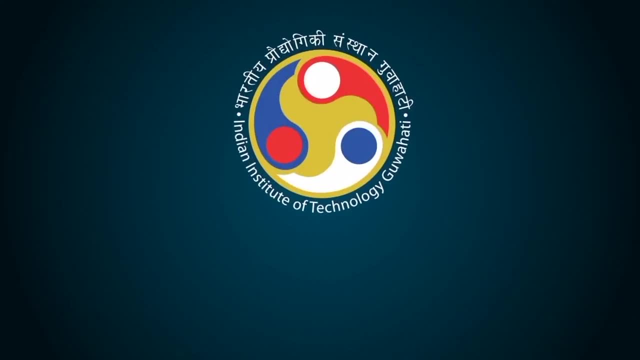 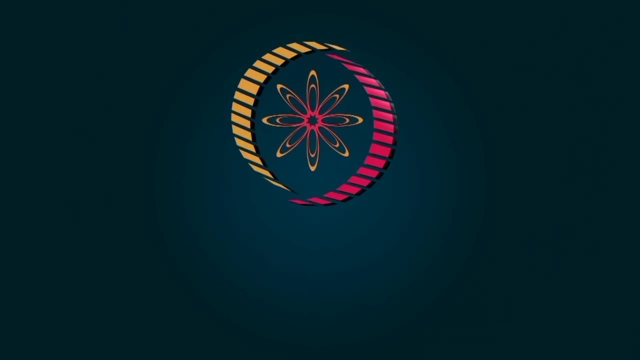 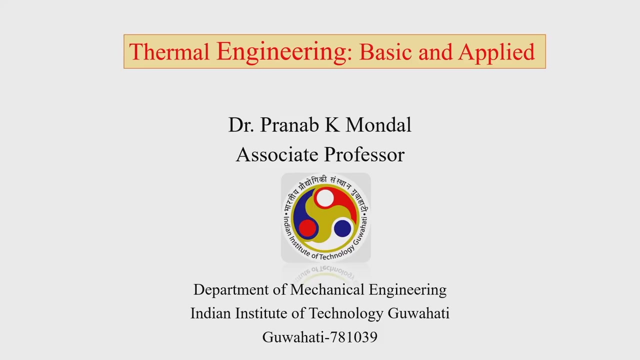 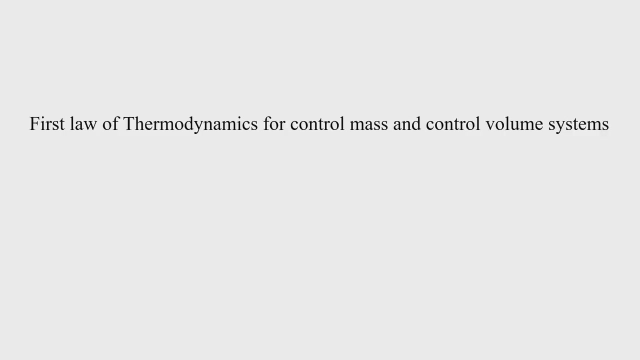 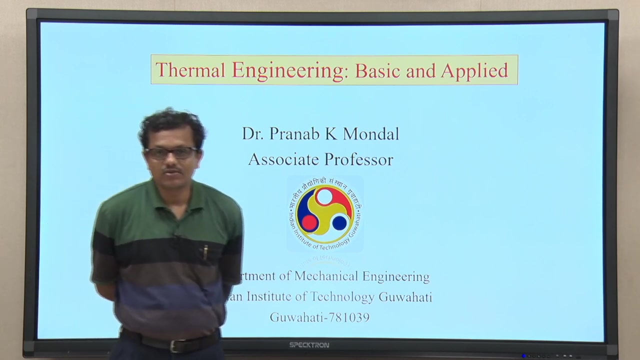 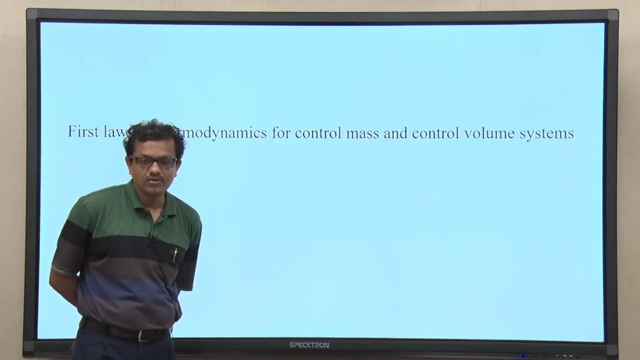 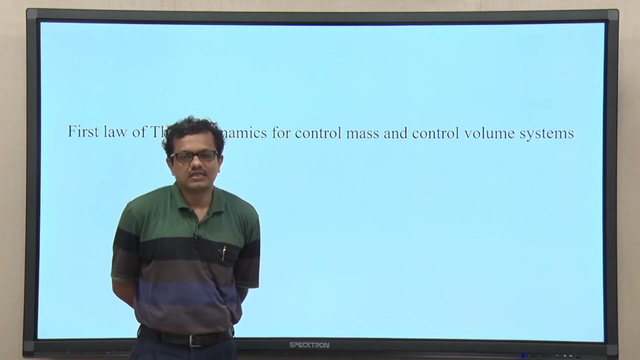 Thank you for watching. I welcome you all to the session of thermal engineering and in today's class we shall discuss about the first law of thermodynamics, applied to both control mass and control volume systems. You know that in this course, as name you know suggest we shall be discussing about 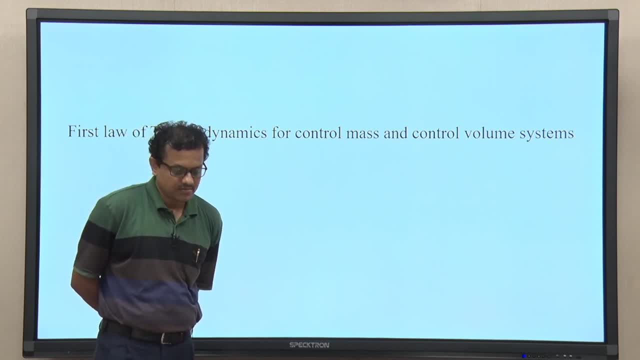 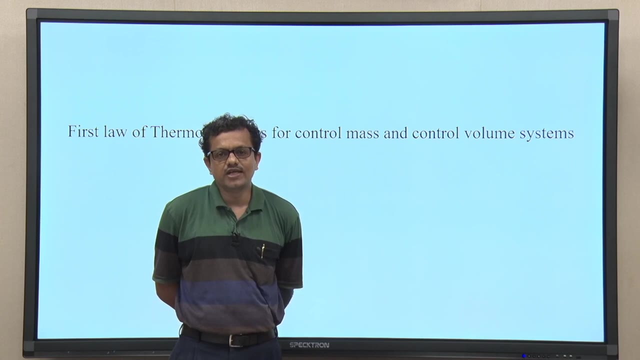 the thermal engineering systems, essentially to learn the analysis, also the operational procedure, of different thermal systems. So question is, why do we need to learn all these aspects of thermal engineering systems? You know that for the human comfort, along with the process considering different practical applications, be it power plant or any process industries. 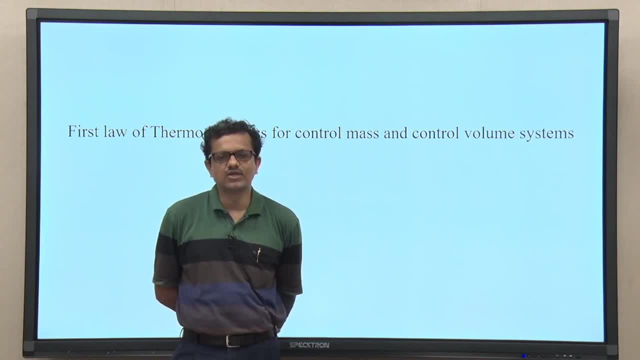 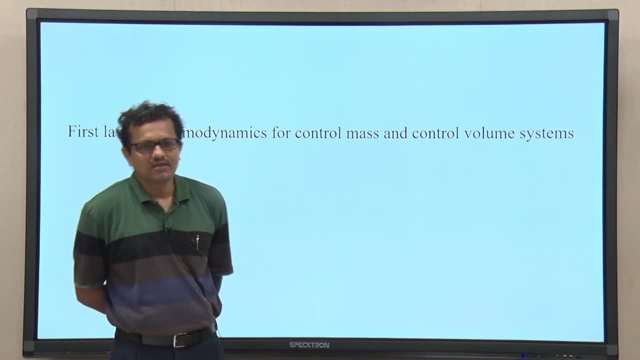 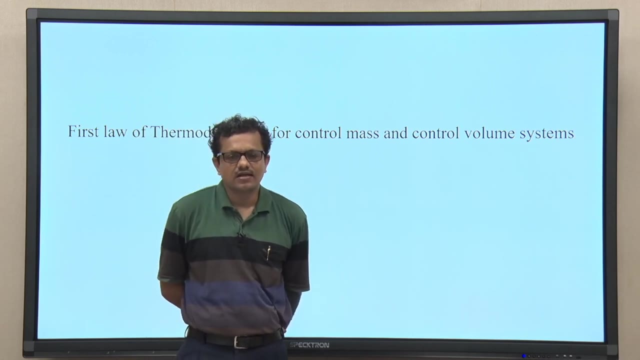 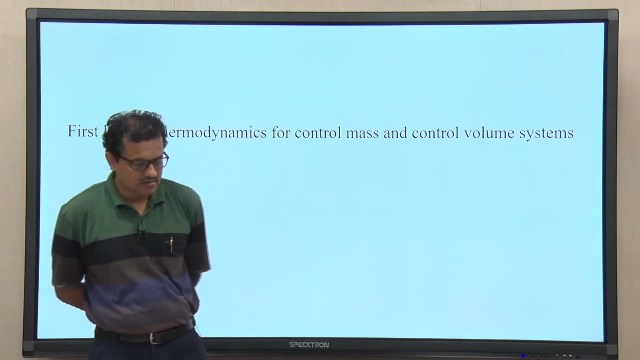 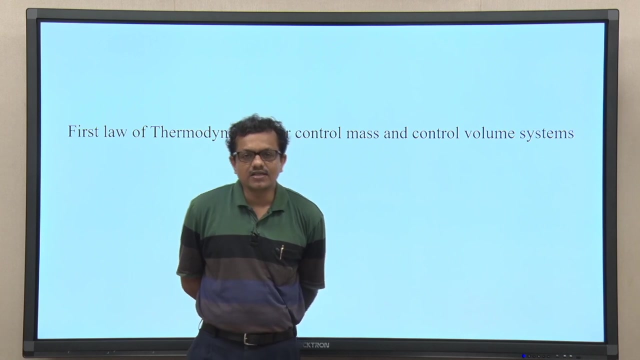 and, as I was talking about human comfort, So you know air conditioning as well as refrigeration system. in all these systems you know whatever processes are there. If you need to learn those processes, we need to understand about the thermodynamics, also the fluid mechanics. Now, by learning the basic things which will be applied to understand 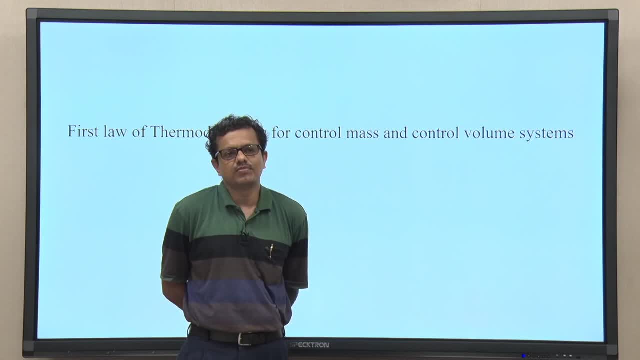 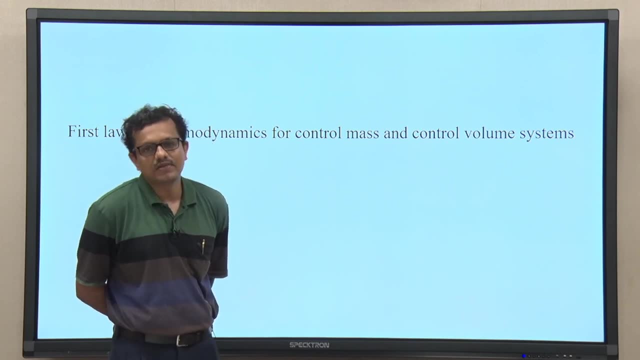 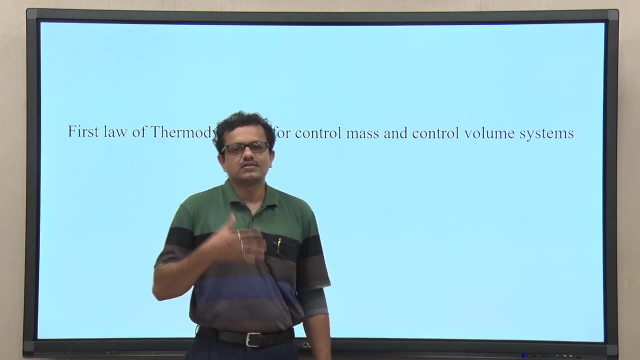 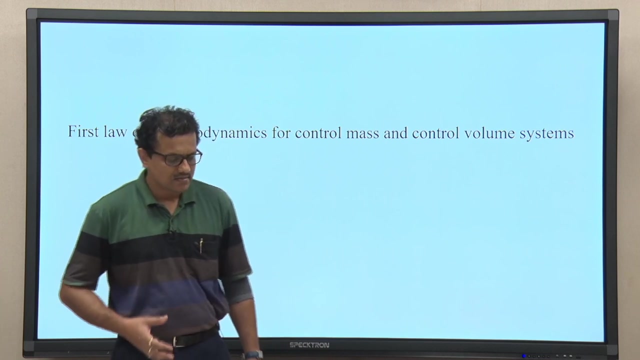 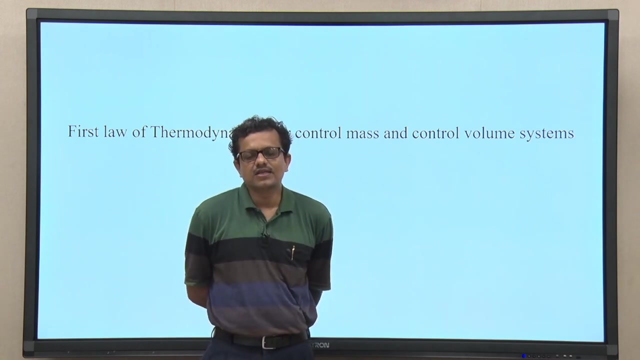 the overall performance overall. you know, analysis of the system is very important to the designer, at least to have a good understanding of the system. So that is what we are going to discuss today. I have in today strange help. It is very easy to give the basic concepts Some paper all ticking, some teenage methods. 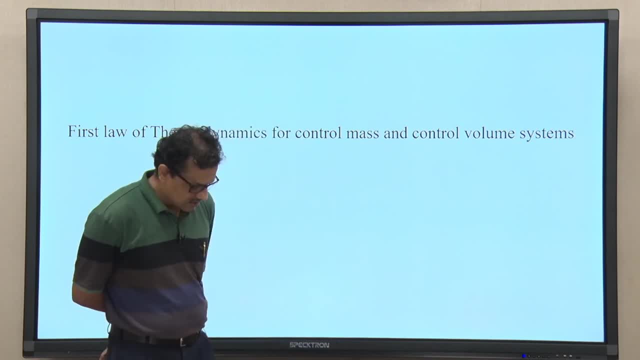 THEMEar task in you know theseiedz is- I am using something, The usual self-allows mày learning topics, The general concept of facts, monuments, gradientsراining, dashing and other questions related to the bad to solve fewishna parable, which you must have as much as possible. 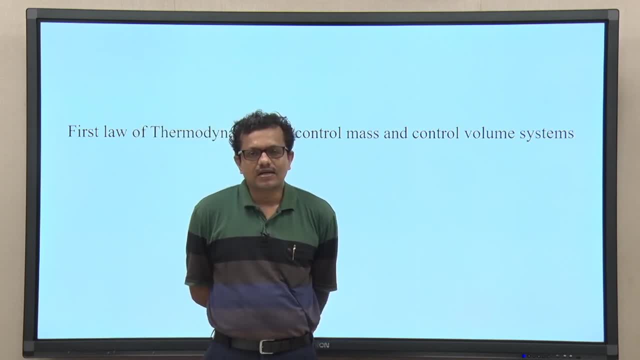 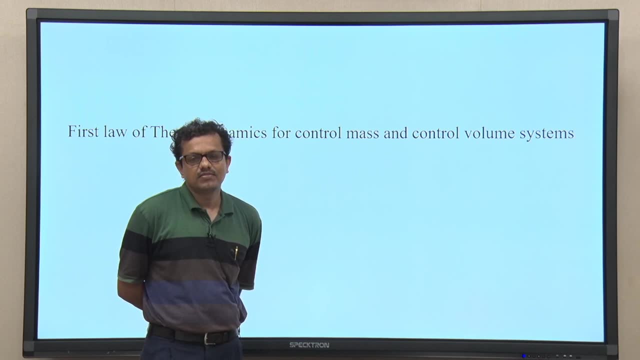 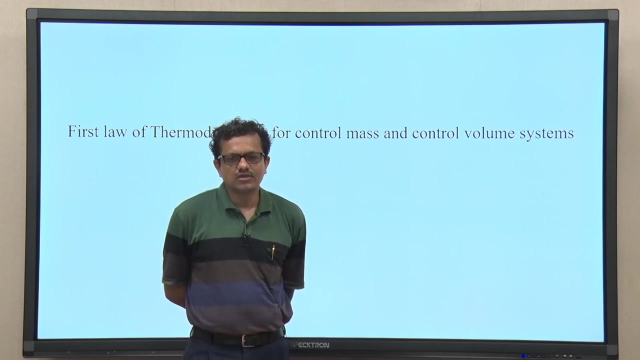 Screen collation of text. strike су éíre个. you know applied part, but to understand the procedure and analysis of those applied system in a greater detail, I was thinking to discuss a little bit about, you know, the thermodynamics, basic of thermodynamics, like first law and second law, So the combination of these two laws are 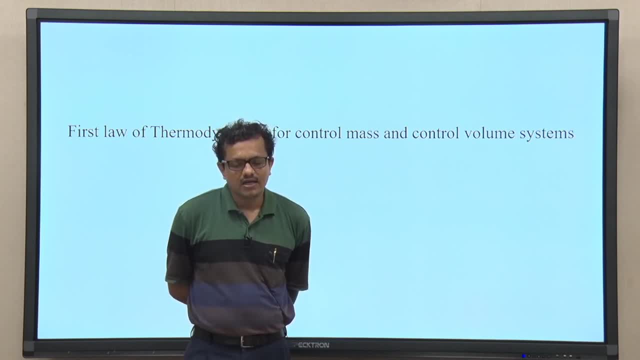 important and if we need to apply, if we need to know the, rather, if we need to map the processes in different thermodynamic planes, essentially to estimate the performance of those processes, we must know the combination of first and second laws applied to different processes. 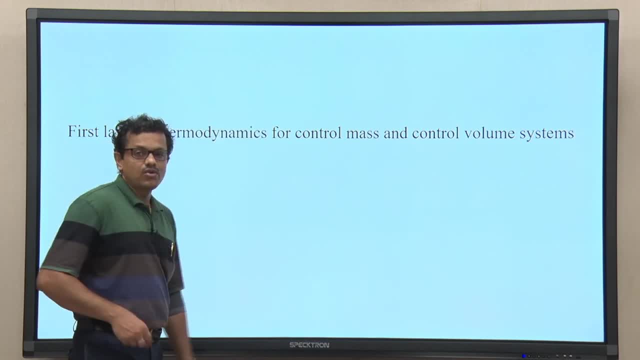 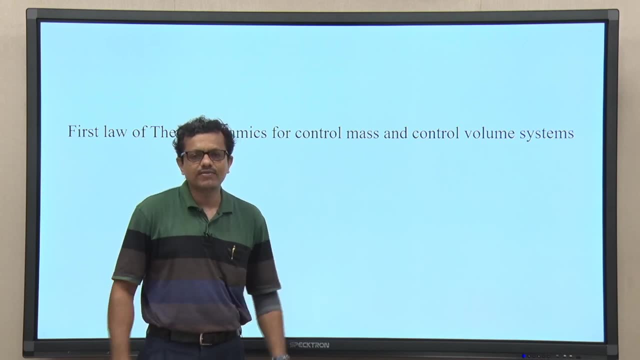 So, to start with today, we shall discuss about the first law. in fact, I am not going to discuss in detail about first law, rather we shall translate. So let us try to recap whatever we have learnt from our basic thermodynamics course. So 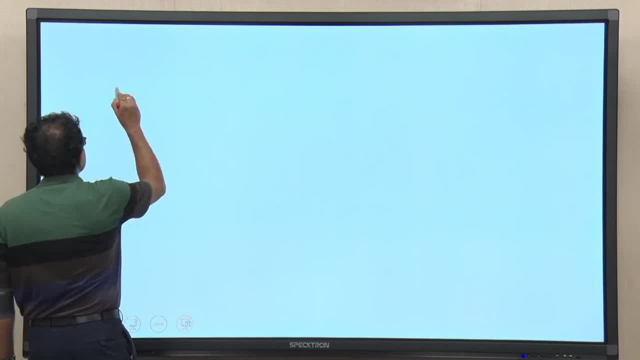 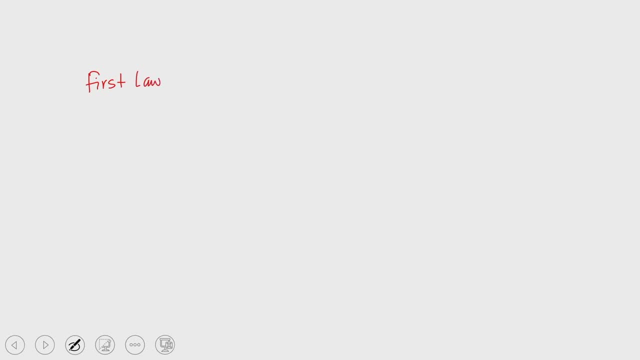 you know that we have learnt about first law of thermodynamics. So first law of thermodynamics, first law of thermodynamics. So today you shall see that if we try to apply this first law for the control mass as well as control volume system, what would be the form of the equation And what are 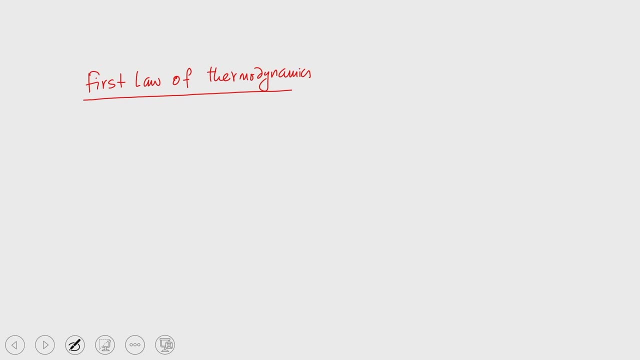 the different forms of the equation we shall try to establish because these equations will be very much, you know, useful to understand the processes in different thermal systems. So if we try to apply first law for the control mass system initially, Then we understand there may be stable professional thermal systems but for this thermal system itself may be. 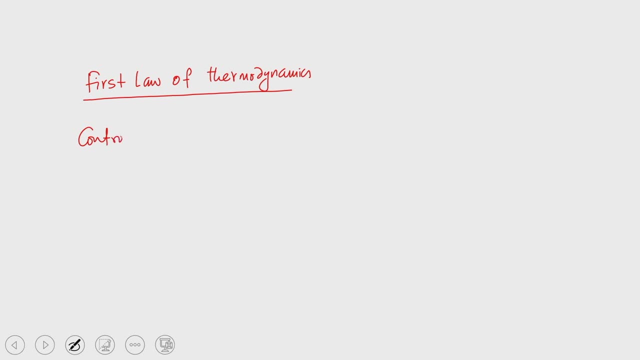 not stable if a field is integrated with a flow stream in it. we can try to understand those matching times for the combination of dec εκ terms. and what is the difference between guys? So this is control mass system. What is control mass system? We have seen that there is no. 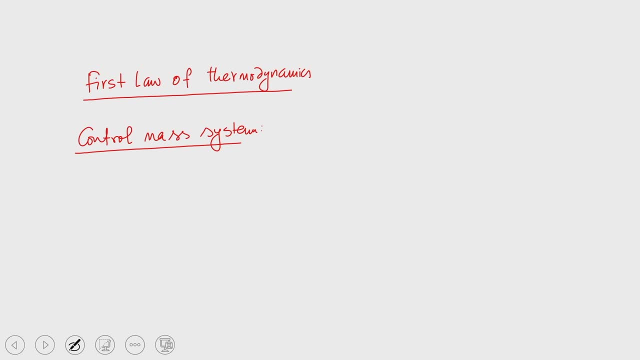 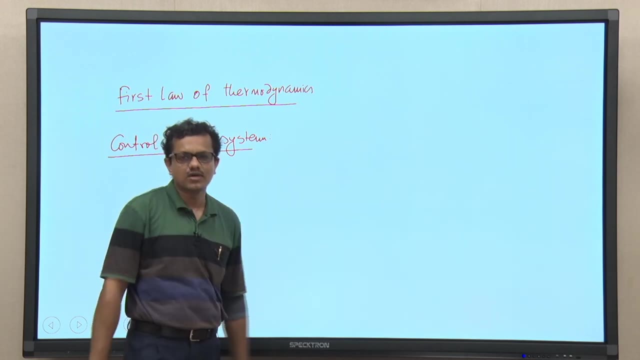 interaction of mass with the surroundings. Even if we allow that. we have learnt from thermodynamics course that even if we allow that a system, so if the mass in is equal to mass out, So at any time we can see that the mass is remaining fixed. but in that case 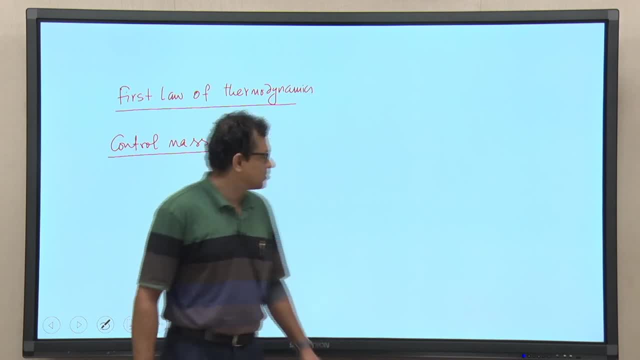 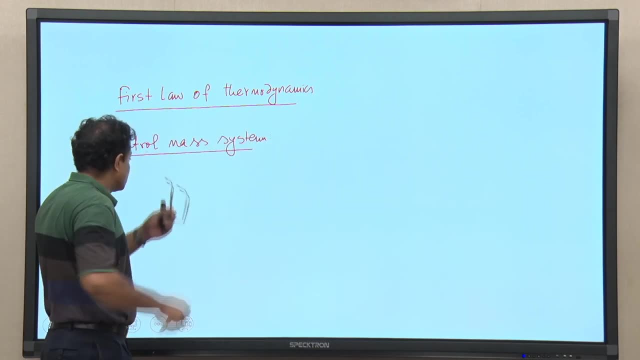 identity will be changed, So we cannot call it as a control mass system. So control mass system, that is, there is no mass interaction with the system, rather between system and the surroundings. So now, if we try to apply the first law to the control mass system, 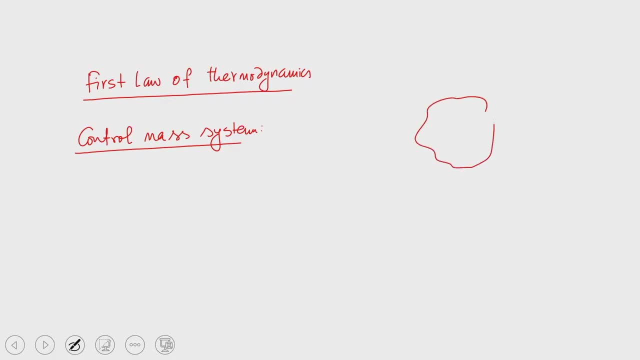 we can consider a control mass system any arbitrary control mass system, lumped system, So this is a lumped you know system And or lumped body and if we have, so this is control mass system. Now we will be applying, rather we shall try to understand if we apply, if we try to apply first law to the system. 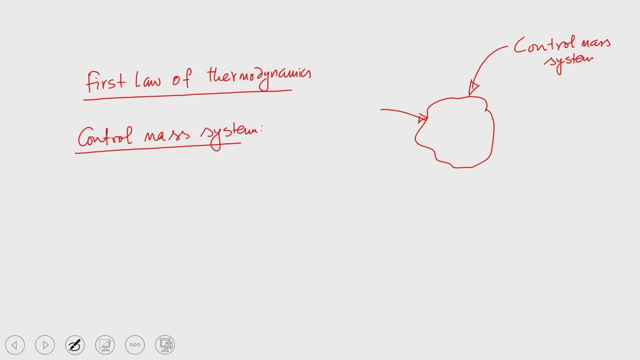 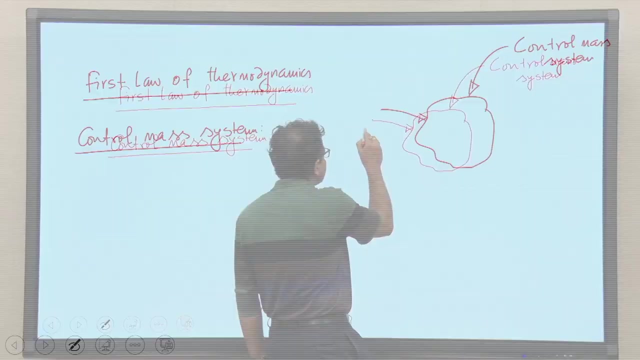 what would be the equation, mathematical form of the equation. So what you know, what we have learnt from basic thermodynamics course, is that first law is the statement of energy, statement of the conservation of energy, to be precise. So, if we consider, this is a control mass system and energy input is E in and from the 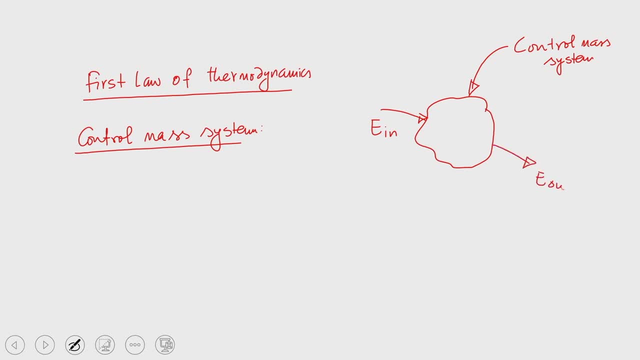 system energy output is E out, then from the conservation of energy you can write that you know E dot E in minus E dot out. So we are trying to write this in a rate equation plus something equal to D e by D t, right? So the this is: 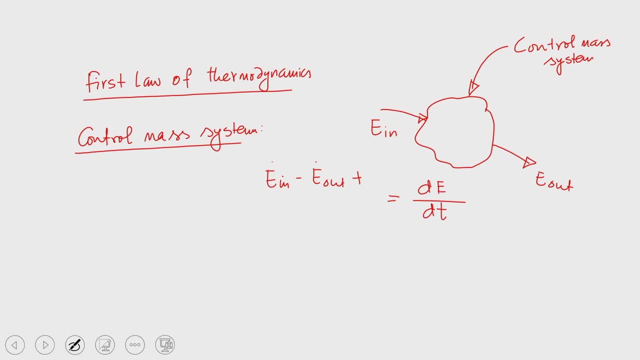 D e by D t. So this is for system right. So the energy input of energy at which the rate at which energy is entering into the system minus rate at which energy is leaving from the system is nothing but the change of energy within the 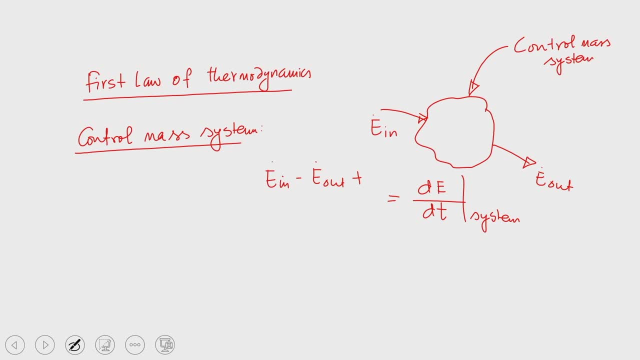 system. Also, we need to take into account one important term, that is, energy generation. there might be some ways by which energy may generate within the system, and that is why we have taken this particular term right Now. question is: till now we have talked about. 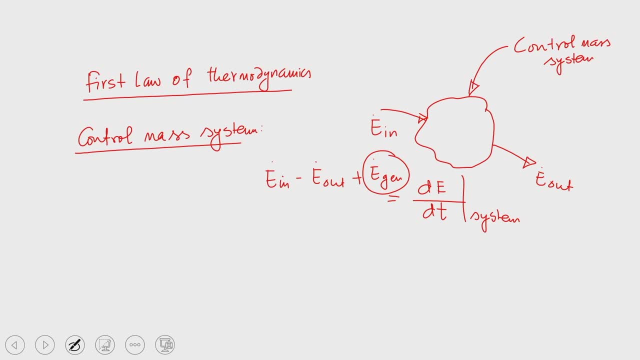 the energy change. So if we try to write this equation for a particular process, say, we are trying to apply this equation for a process in which there is no energy generation. So right Now question is: why we have taken this particular is why, when we can consider that there is no energy generation, we are assuming that 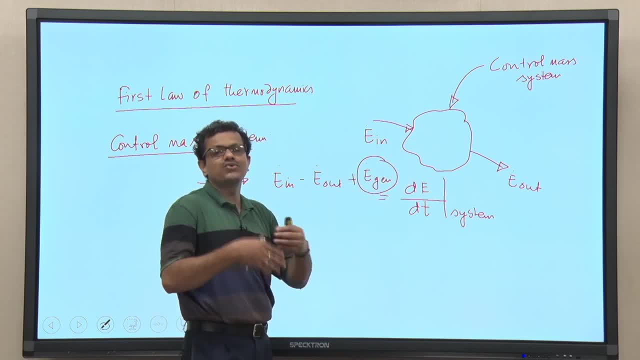 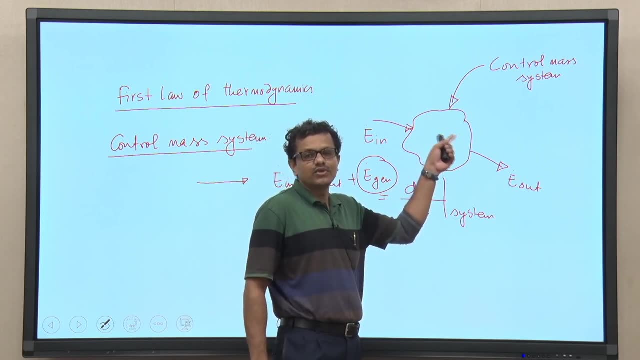 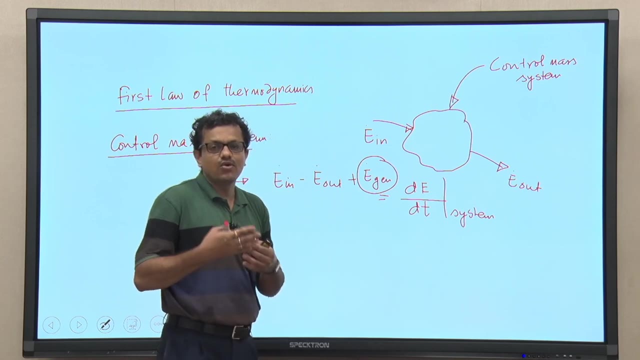 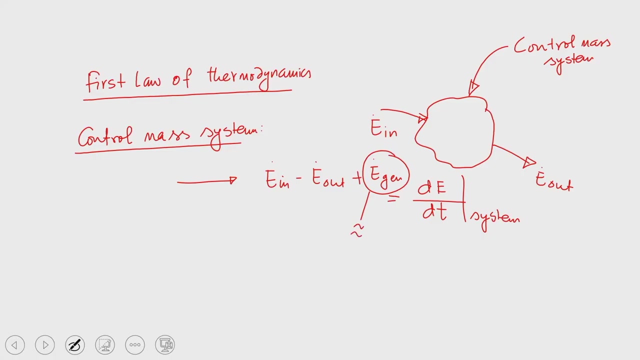 energy interaction with the system is only through heat and work. So energy interaction of the system, that means energy interaction of the system with the surroundings. So when the interaction of energy between system and surroundings is only due to the heat and work interaction, then this term can be 0. So this is equal to 0. So we are writing here: 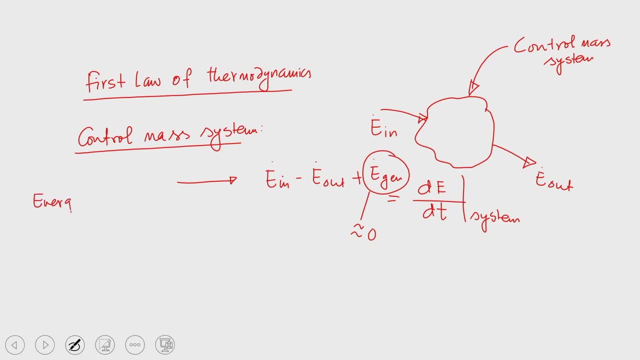 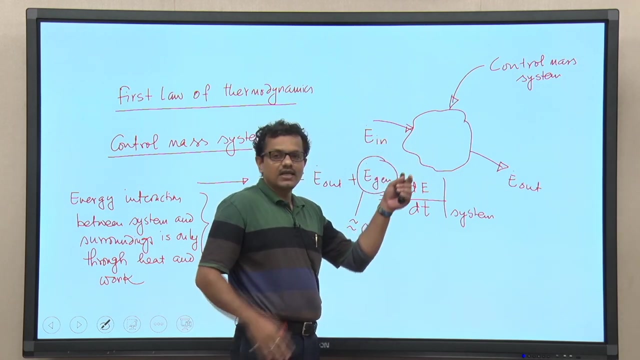 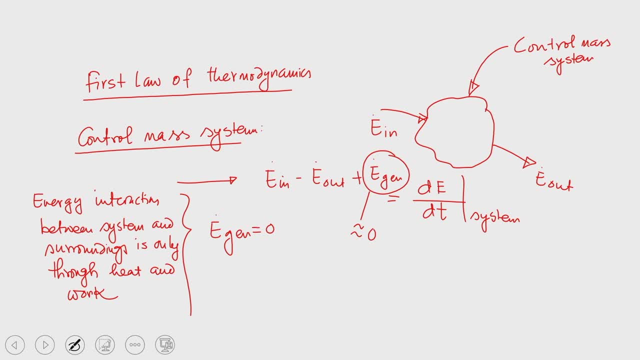 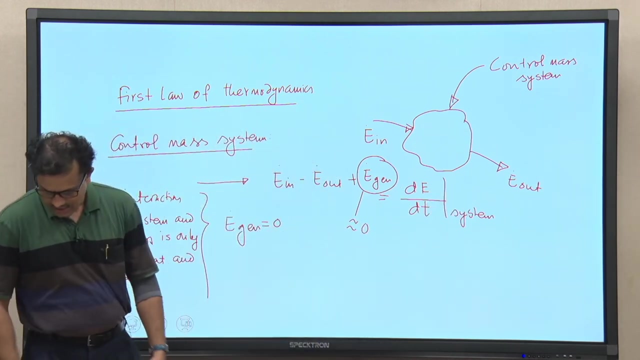 surroundings in the form of heat and energy interacting between system and surroundings in the form of work. if these two forms are there, then there is no energy generation. So this is the energy. you know change within the system. Now question is: so you can assume 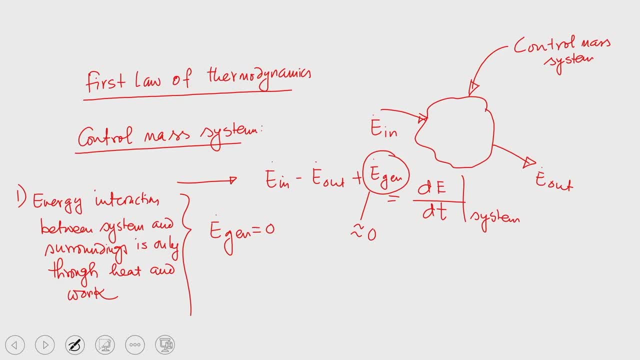 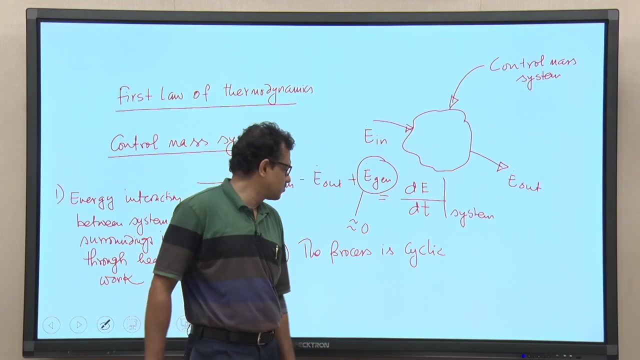 this is one assumption, and if you also can consider that the process is cyclic process, So the process is a cyclic process. So I am not going to describe this because you have learned about the processes: different processes, Reversible process, irreversible process, cyclic process- so many processes. So if the 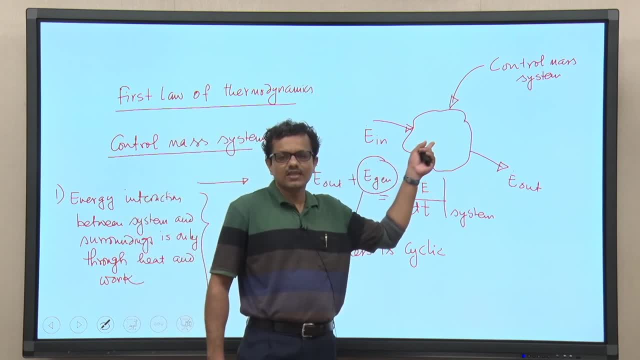 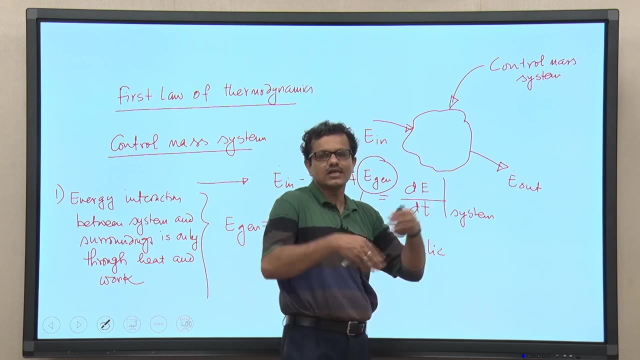 process is cyclic. that means we can restore the system. I mean if we try to give some energy input to the system, then after certain time- may be after interaction, after having interaction with the surroundings- system can be brought back to the initial state. So this is cyclic. 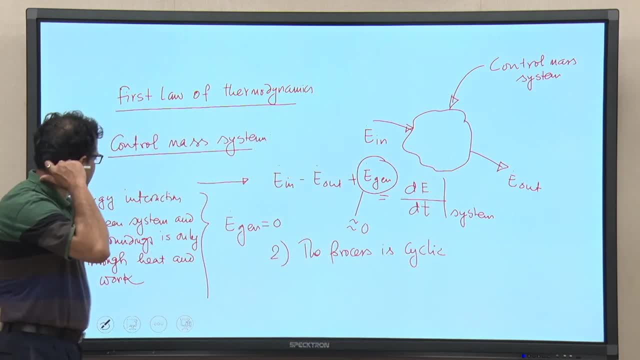 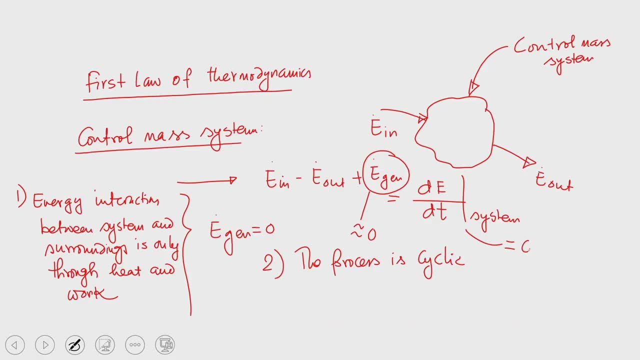 process. So now you know what I am telling you: that if the process is cyclic, then this term equal to 0.. So this is using 2 and this is using 1.. So now, if we try to write this generic form, 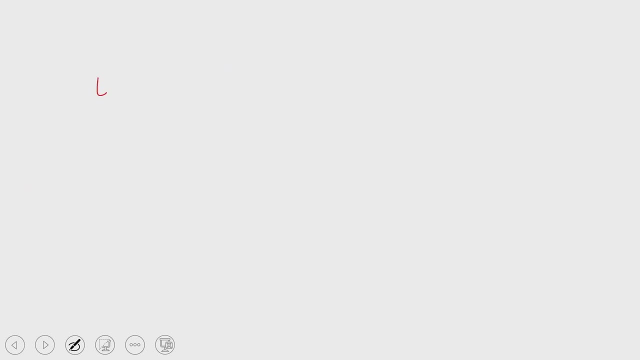 we will be getting e dot in 1.7 nelle by 2 into q. So this is using 2 and this is using 1. 해서 tenemos es understanden This term slightly. different region between system and minus E dot out equal to 0.. What we have discussed? We have discussed that the interaction between 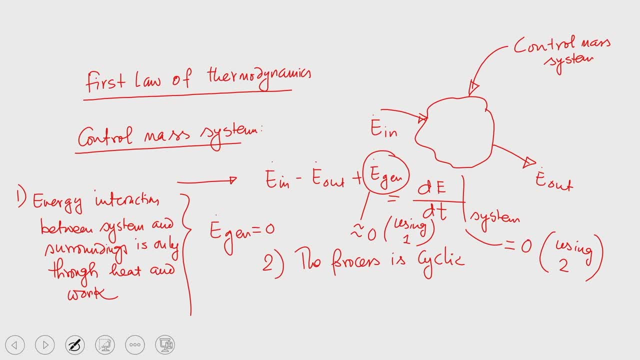 system and surroundings is only through heat and work. There is no other forms of energy which is either entering into the system or transferred from the system right. So there is except heat and work. there is no any other forms of energy which is either entering to 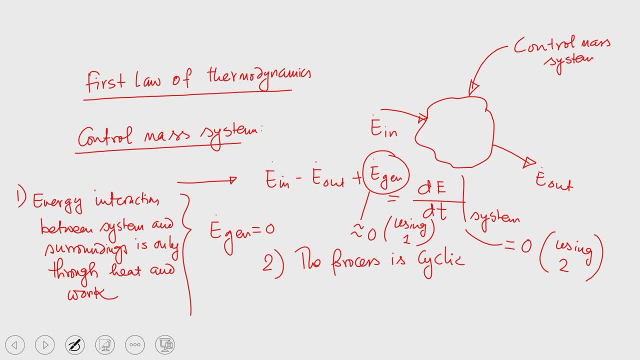 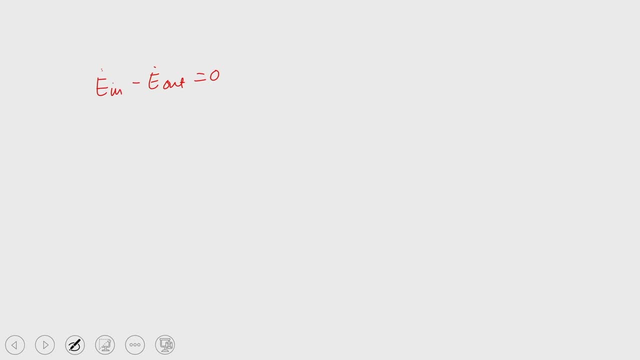 the system or leaving from the system. So if that is the case, you know we have learned from thermodynamics that in it is, you know, mostly followed that energy transfer by heat is taken positive. So energy transfer by heat to the system is taken positive. 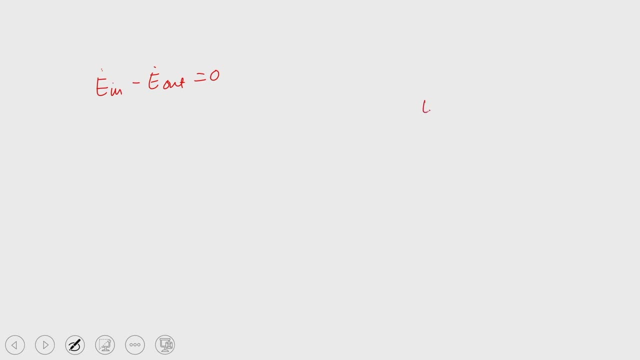 So let us write over here that energy transfer by heat to the system is taken positive. So when there is heat transfer to the system, that is positive. that is the you know keyword. and now, if the energy is transferred from the system following this notation, it should: 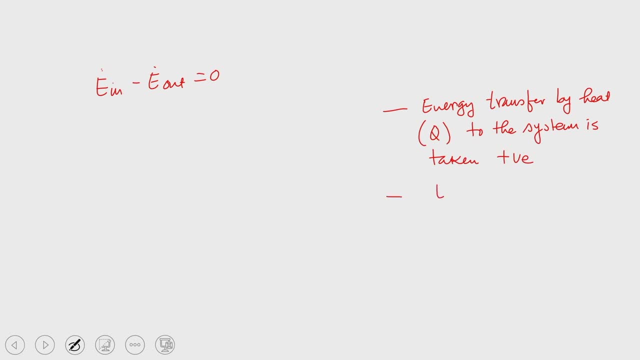 be negative: okay. In a similar way we can write energy transfer by work: Okay. So energy transfer by work from the system is taken positive. So that means if some amount of work is added to the system, it should be negative. So, following these two, 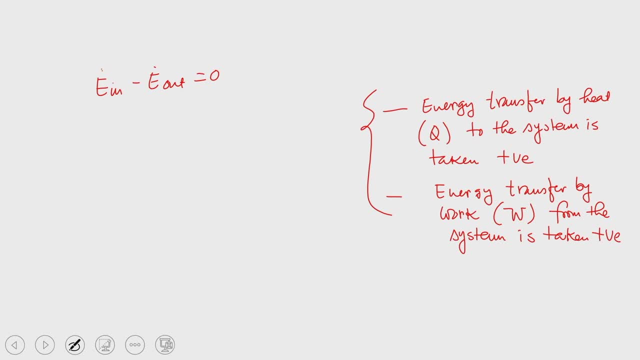 notation. following these two notations, which is which are largely followed, you can also consider reverse, but accordingly you have to consider for rest of the analysis. So if we try to write it, we can write that q dot minus w dot equal to 0, right, Because 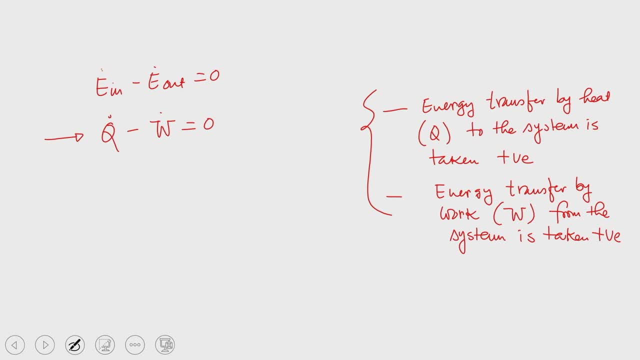 only energy interaction between system and surroundings is equal to 0,, right? So if we write it, we can write that q dot minus w dot equal to 0, right, Because only energy interaction between system and surroundings is equal to 0,, whatever frequency is obtained. 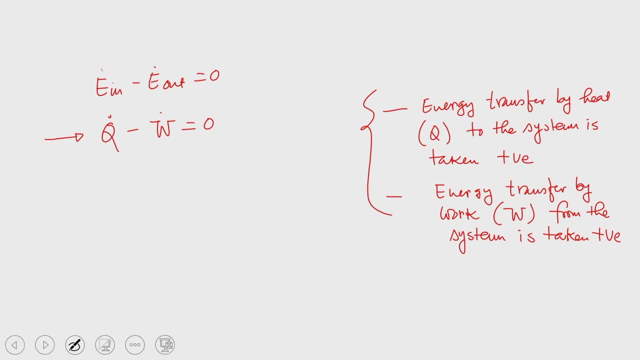 from the system, it becomes negative. So this is the rate equation. If we try to write a total, so this is the rate form, this is in the form of rate equation. So what would be total? So if we integrate it over, 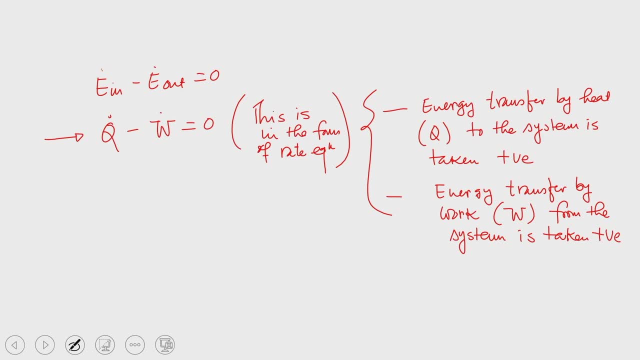 cycle over time, then we will be getting the total. If we integrate it in a cycle over time, then we will be getting the total. So if we try to write it, then delta cube minus delta w equal to 0. So if we integrate it over cycle, over time, then we will be getting. 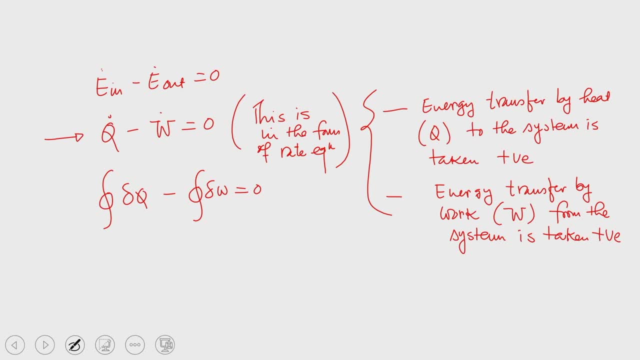 total. So this is the equation, and if you try to write cyclic integral del cube equal to cyclic integral del w, So if you try to integrate it over cycle, over time, we will be getting this equation, And this equation which is very famous perhaps. 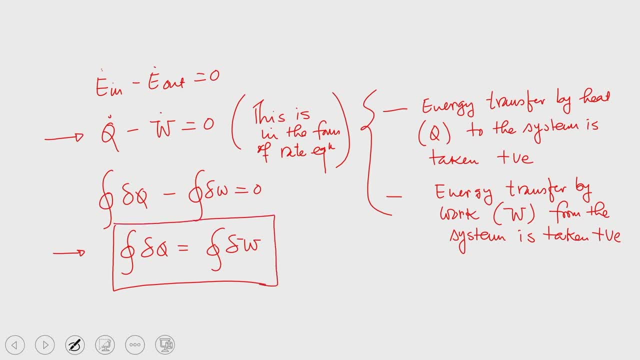 you have Studied this, you can easily identify it. So this is first law of thermodynamics for the control mass system undergoing a cyclic process. So, starting from the generic form of the energy balance equation, we have established that the first law for a system undergoing through a cyclic process can be written in: 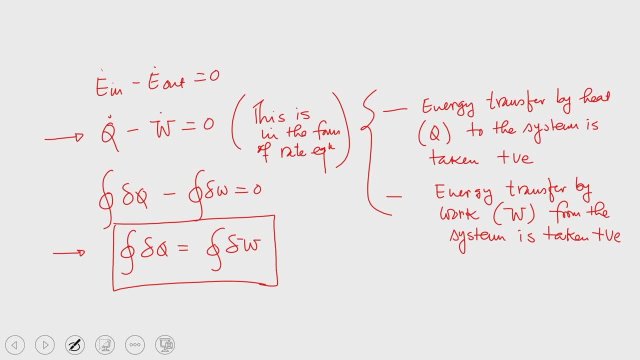 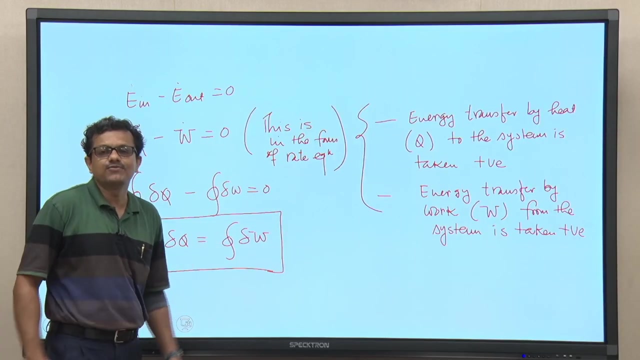 this form. Now what we can tell from this equation? perhaps you have read, you have, you know, derived this expression in thermodynamics course. So basically, you know that this equation indicates that if we supply certain amount of heat to the system- I mean energy, but in the form of heat- the system has capability. 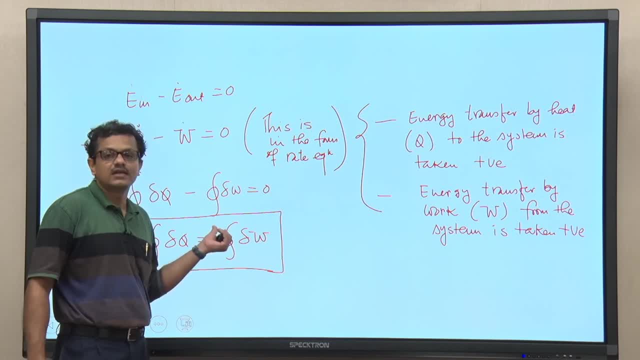 to do some work. That is What this expression tells us. so this expression tells us that if we supply certain amount of heat to the system, system has the capability of doing certain amount of work. So that is the take home message you can take from this expression. 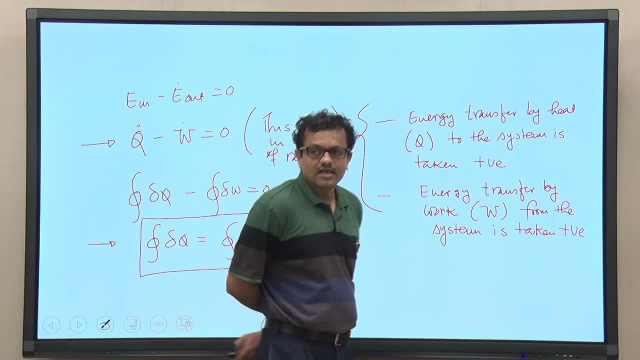 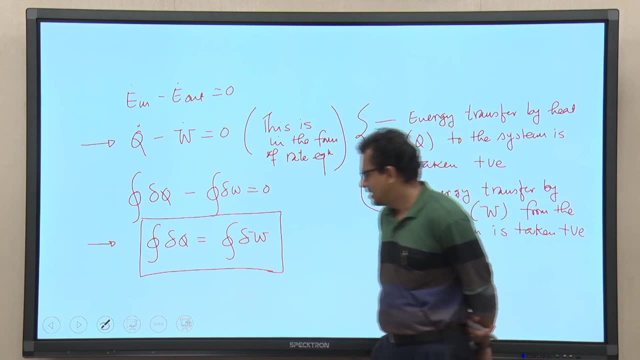 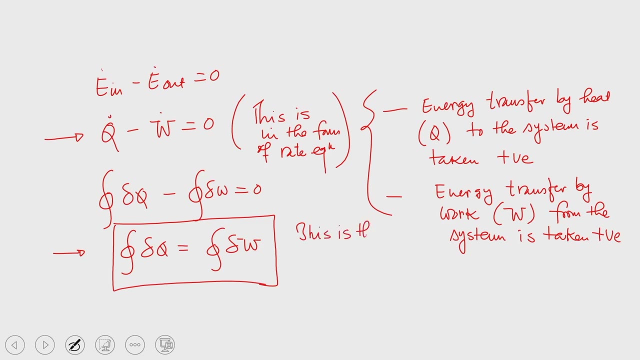 So this is basically the expression of first law of thermodynamics applied to the control mass system undergoing the cyclic process. Let us write so: this is: This is the first law of thermodynamics for the control mass system undergoing the cyclic process. So first, the first law of thermodynamics for the control mass system undergoing the 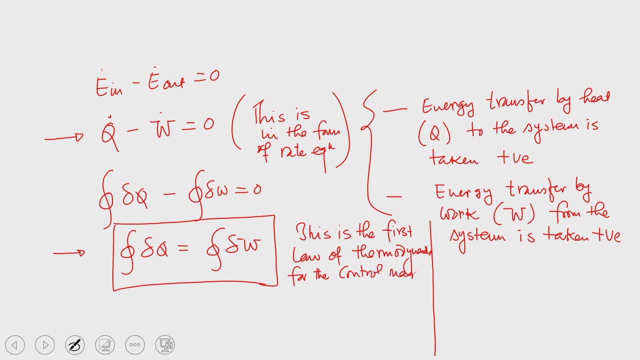 cyclic process is recorded, So let us write. So this is undergoing through a cyclic process- I am underlining these two words. that is, cyclic process. If the process is not cyclic, then what will be the form of the first law? even? 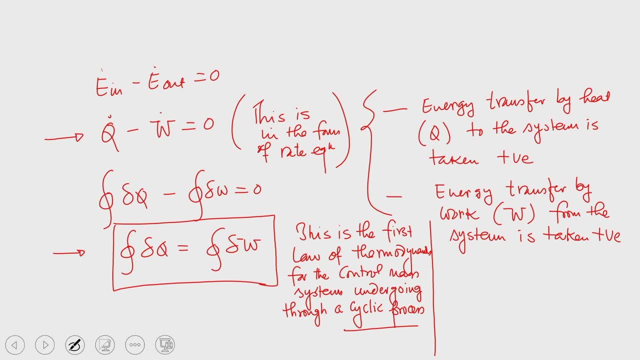 if we apply for the control mass system. So this is very important. you know that we can write the first law, even for the control mass system, but if the process is not the cyclic process, It is quite obvious that all processes will not be the cyclic process. So if we need to write the expression for the similar 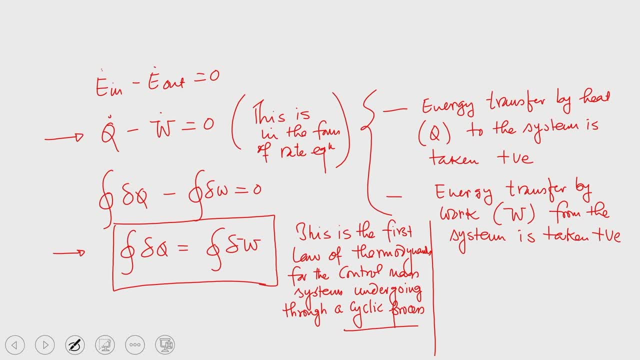 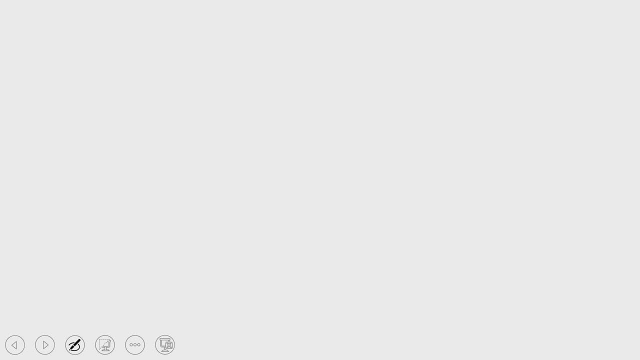 such expression for the general processes. what would be the form? So fine, now we will be. we are discussing the first law for control mass system. So this is a general process undergoing through a process which is not a cyclic process. This is a general process. 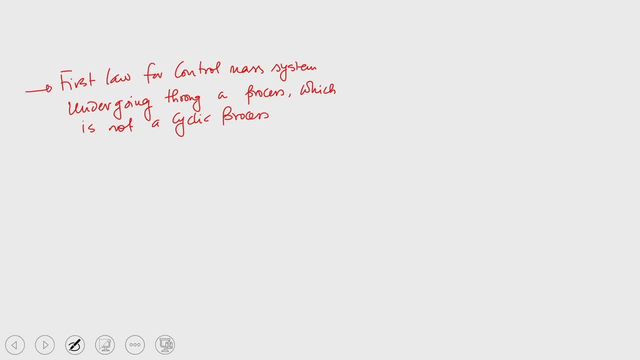 Video Lecture on Experimental Stress Analysis, Prof R Ramesh IIT Madras. Lecture on Experimental Stress Analysis, Prof R Ramesh IIT, Madras. So this is essentially our objective is to derive the equation when the process is not. 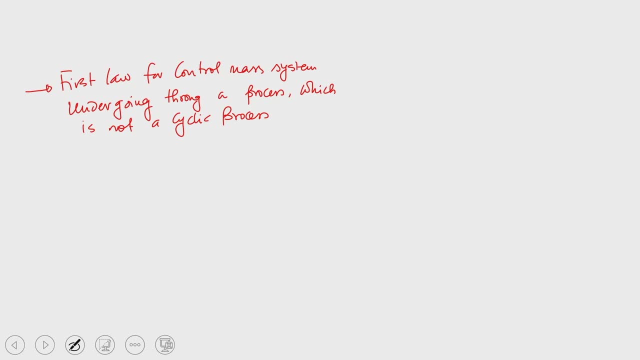 a cyclic process. In other words, we shall take an effort to establish the first law for the control mass system, when I know process is any generic general process. So you know that if we try to say we know so, if this is the process, if this is the control mass. 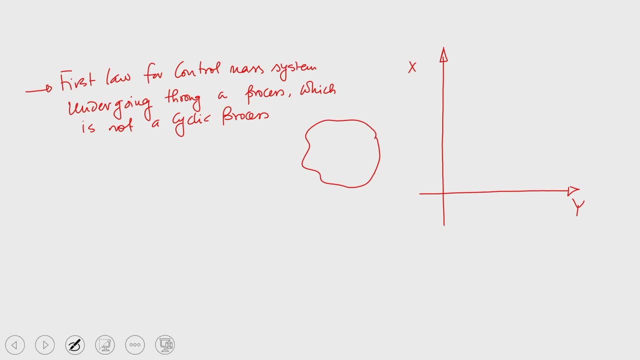 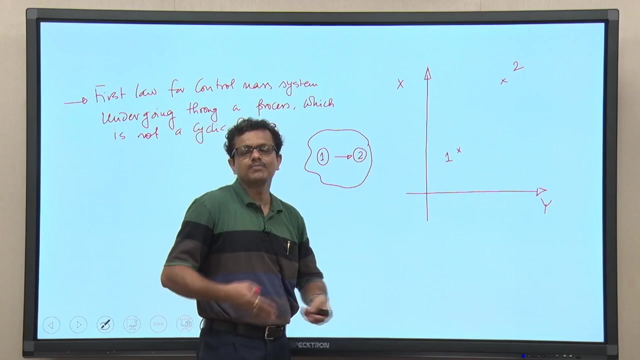 system and the system is changing its state from state 1 to another state 2.. So this is the control mass system and the system is changing its state from state 1 to state 2, but not following a cyclic process. It may be any other processes, So if that is the 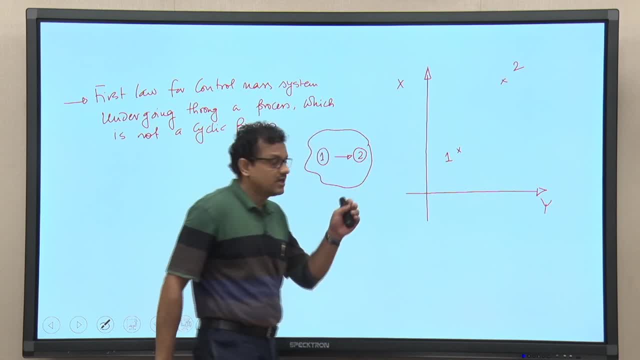 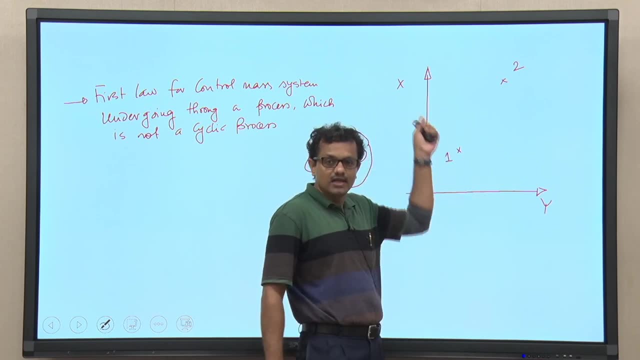 case, we are trying to map that process in this thermodynamic plane. we really do not know what are the different properties, x and y, why It may be temperature entropy, it may be pressure volume, it may be enthalpy entropy. 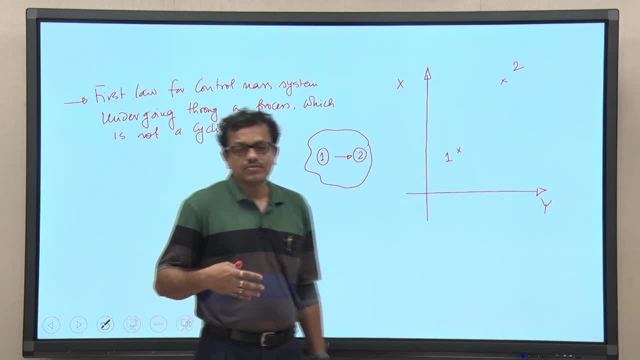 So mostly in this course we need to map the processes, rather different thermodynamic processes in different thermodynamic planes. What are those planes? Pressure volume, pressure temperature volume temperature temperature entropy, enthalpy entropy. So you know that I am not going to. 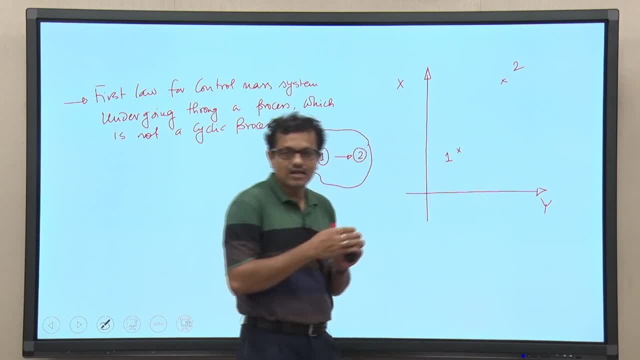 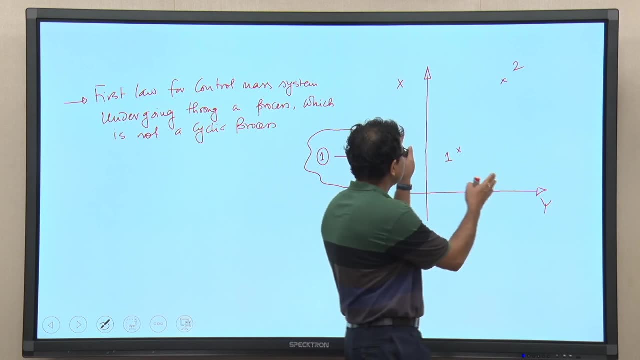 discuss in detail because you have learned it from the basic thermodynamics course. but for today, for the sake of completeness of the analysis, I am considering a plane that is x- y. So these two properties again are generic. we really do not know. Maybe x is pressure, it may be volume. 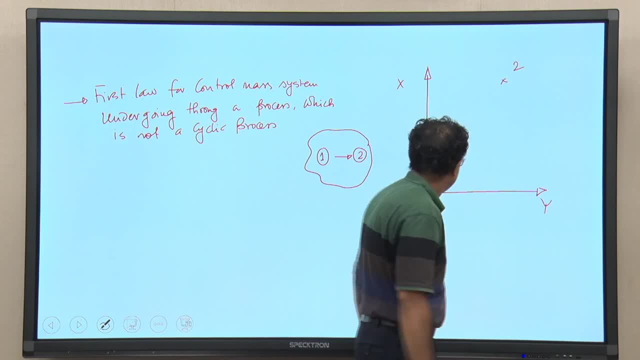 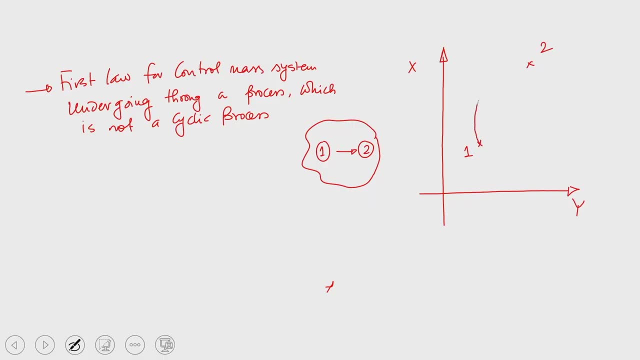 y may be entropy, it may be temperature, like this. So now, when the system is changing its state from 1 to 2, say, it is changing the state from 1 to 2 like this, And it is changing its state from 1 to 2 following this path A and coming back to the same state. 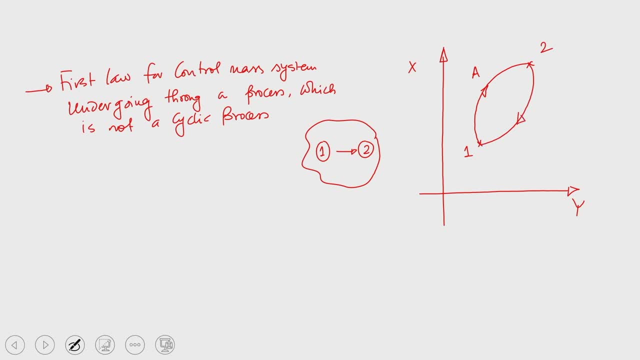 may be following this path B. So basically, you know that we are. if we supply heat to the system, it will, as I told you, that it has capability to do some work. So we are left with the following. we can say: there is because of identity. we have been 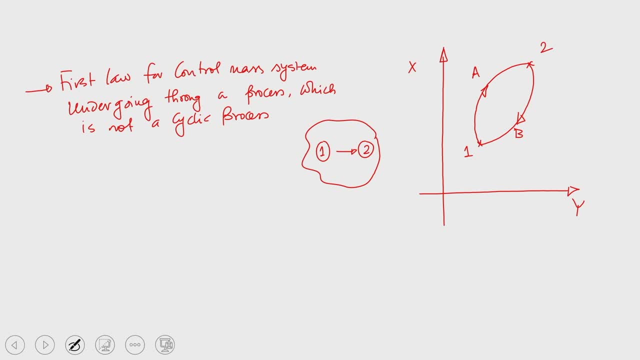 showing that if we supply heat, we get the result like this and Taliban, in our case, is going to have thisome kind of silence. Similarly, we check this sta. we mean if we supply heat at some particular point, like 6, so it could be ready to operate or 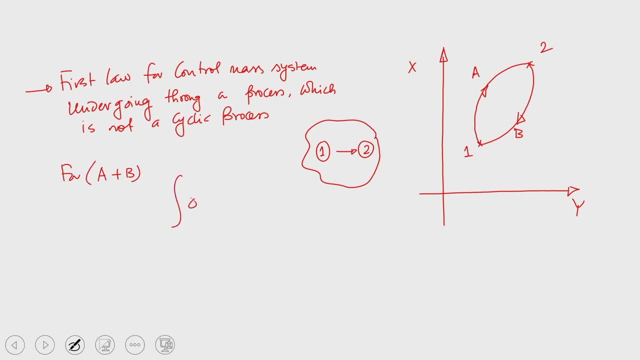 when there is a sudden change到了 2, then it will be like the fine scratching at a particular point. we are not going to decide the state at certain points. The final state wants to say that this is going to be available for dealing down all the two states. So for one example we have. so let us write this plot: 1 A plus B, and we can write del cube: 1 A, 2, 2 A plus 2B and this washing construct in one form as Voice under the canopy. 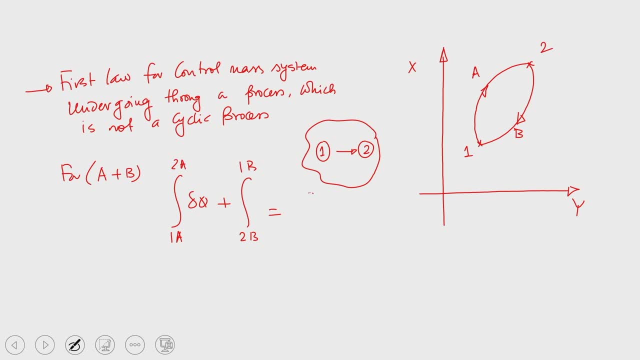 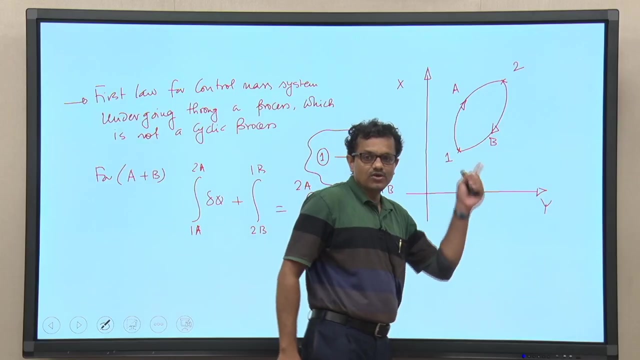 2 b to 1 b, equal to integral del w 1 a to 2 a plus integral del w 2 b to 1 b, right? So that is what we are writing, right, See it is. we know again from thermodynamics that 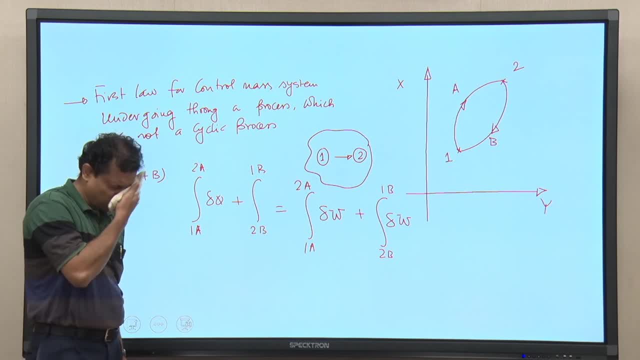 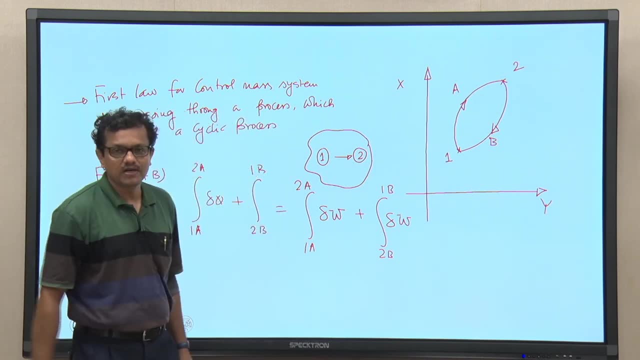 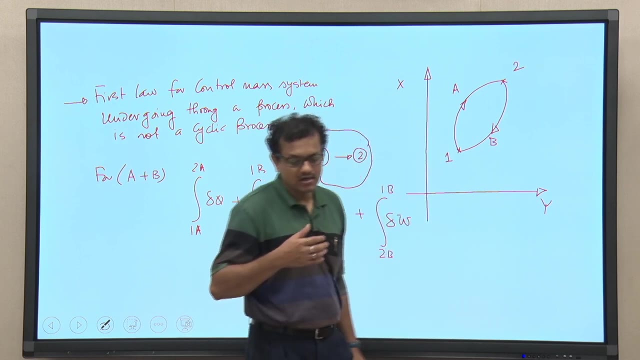 you know this: heat and work, these two are the path function. So these two are not the property of the system. rather, these are the path function. why so? because we have seen that delta w, if we apply, I mean for a control mass system, even if the system is control. 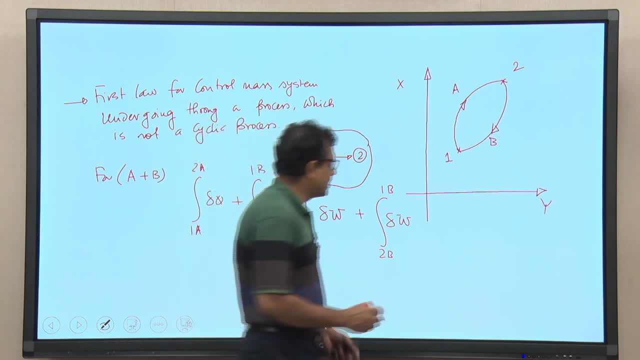 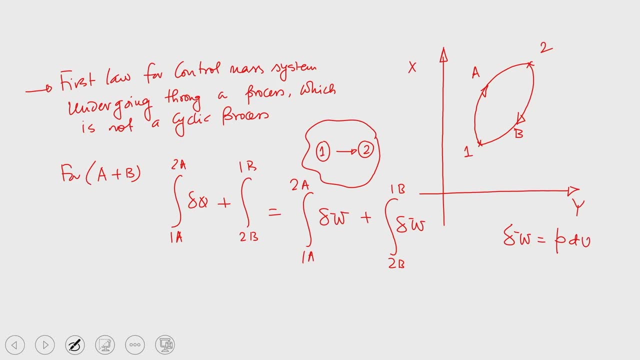 volume system, but if the process is quasi static, we can write delta w. It is not necessary that the system has to be only control mass system. but even if the system is control volume system and but the processes is quasi static process, then it. 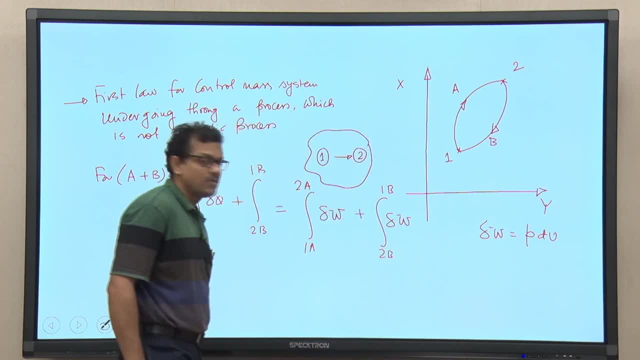 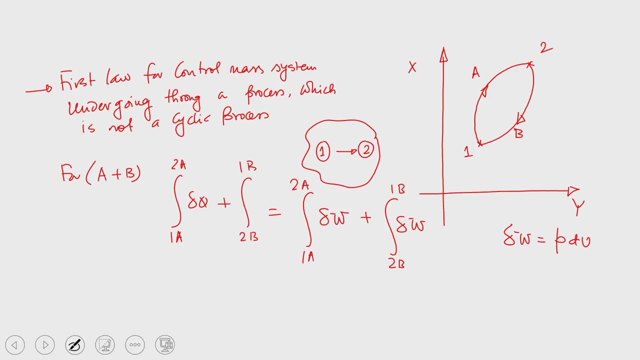 can be written p d v, a simple, compressible, pure substance. Now this you know, understand that this work done is work done depends on pressure and volume. So it does not depend on the straight points 1 and 2, rather the path through, path on which, 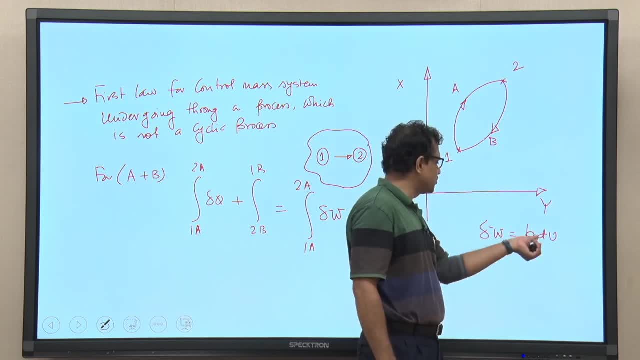 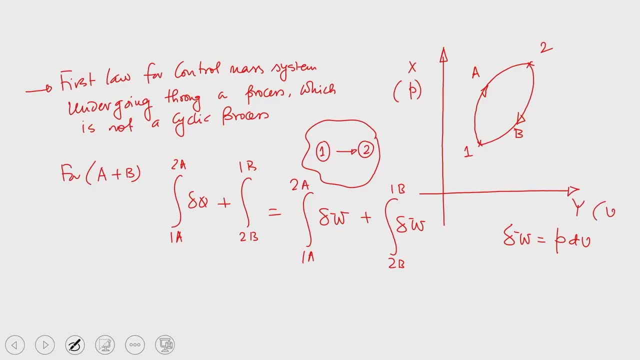 the pressure and volume changes. So maybe the pressure changes with volume. So now, if x and y, so if this is, say, pressure p and if this is volume v. So try to understand if these two properties, x and y, are pressure and volume, you try to understand the change. 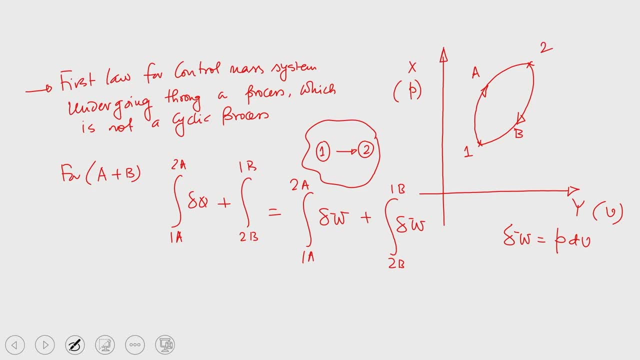 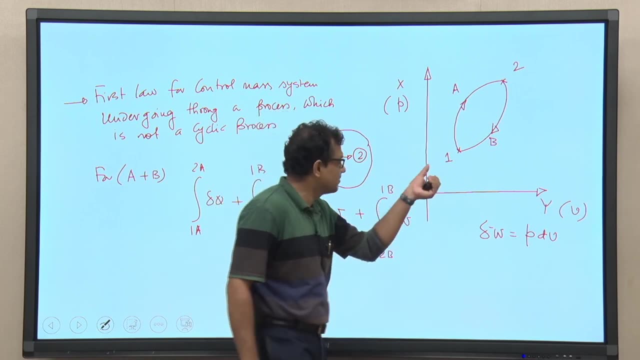 and volume and pressure. following path a is not equal to pressure is not equal to following path B. If that is the case, definitely work done will be different. So this is path function. it does not depend. So the systems is starting from point 1 eventually. 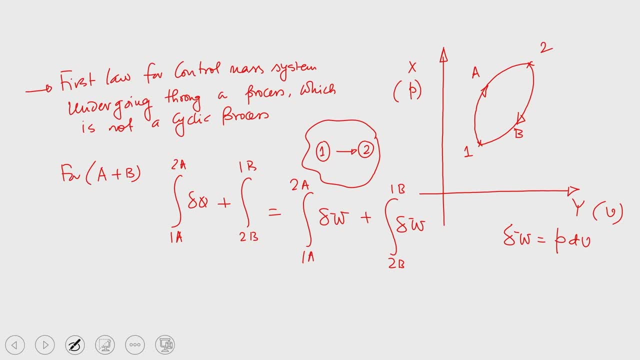 it is coming to state point 2 and it is again coming back to original state. So, but when it is coming to original state it is it is coming through path B. So you know that if we just try to understand the area under the process line it will give the work done. PDB right. So you know. 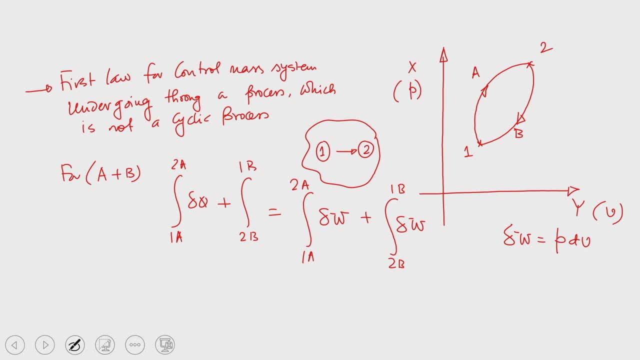 that the change in pressure I mean is I mean the pressure change in pressure and volume, you know, for path A is not equal to path B and that is why these are path function, Though I mean system is coming, I mean system is, you know, the process is taking place between 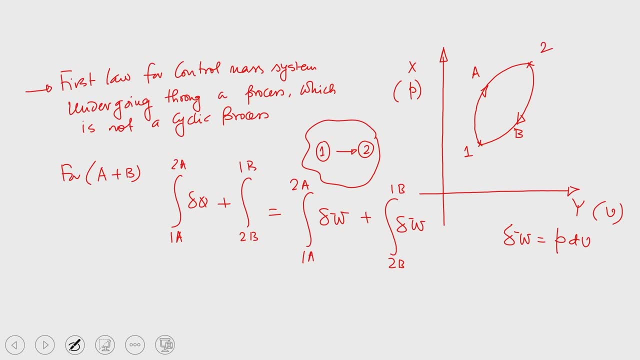 these two state points, but they are, you know, coming back following different path. So this is path function. Also, you know that system is. you know the process is taking place between these two state points, but since these are path function, it is better to write the contour integral. So we are. 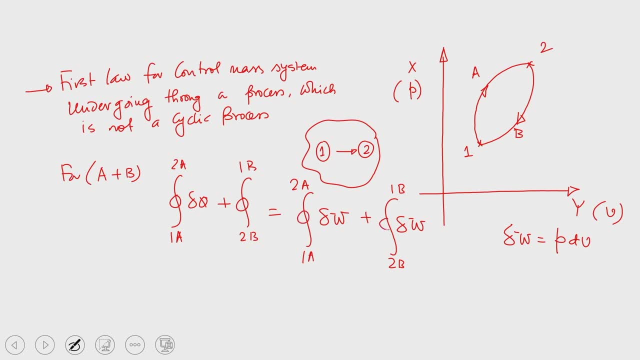 writing like this. So this is not the cyclic process, but since you know this is, you know, change in pressure, I mean work and heat and work, these are path function- it is better to write in the form of contour integral. So now we are considering, since we are trying, 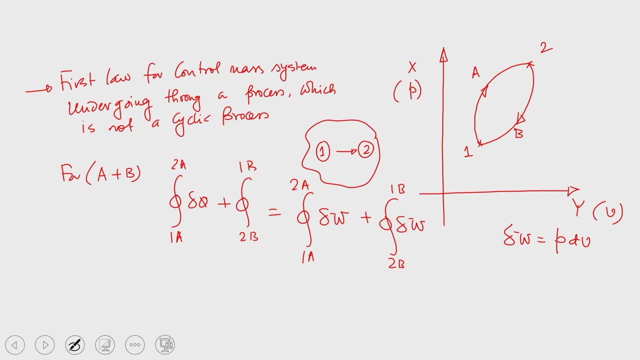 to establish the first law applied to the generic processes, not for the cyclic processes, We are assuming. fine, now, after reaching at point two, system is again coming back to point one following- let us let me write it using different color- System is coming following this path C. So, if so, basically our all of these are. 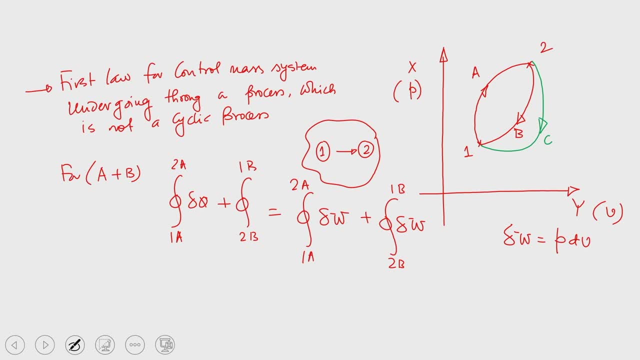 now final. So now same with category first investigator is going to implement it right away. First investigator is going to implement the code that stated in already classes four sets, one final take error. Of course, to explain this we are going to see И gates. 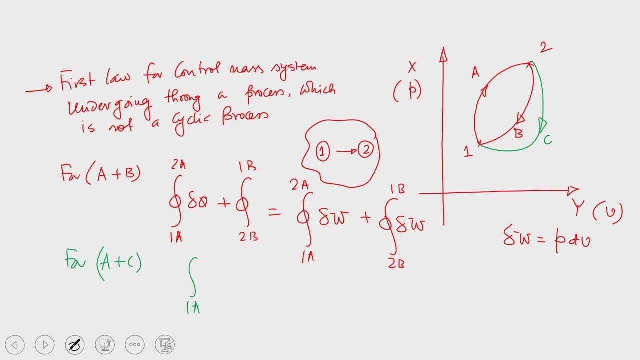 and this is for A gate Furtherwritten code. this code for Cycler set B gates will also be written for C gates. I forgot to write delta q over here, So this is delta q equal to 1 a contour integral, because these are path function. So 1 a to 2 a, delta w, So it is not 2 b again I should write. 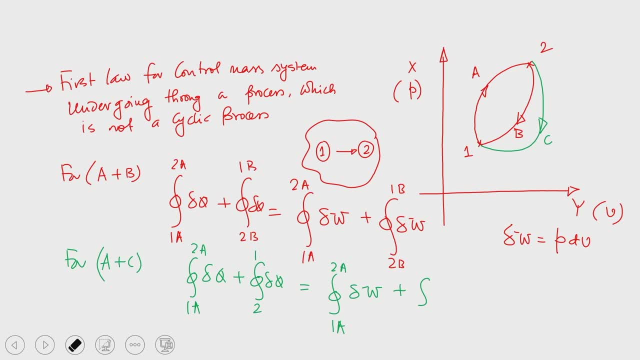 it is 2 c, So it is c, 2 c, and then 2 c to 1 c, delta w right. So this is the expression. So if we give, say this is equation number 2 and this is equation number 1.. So what? 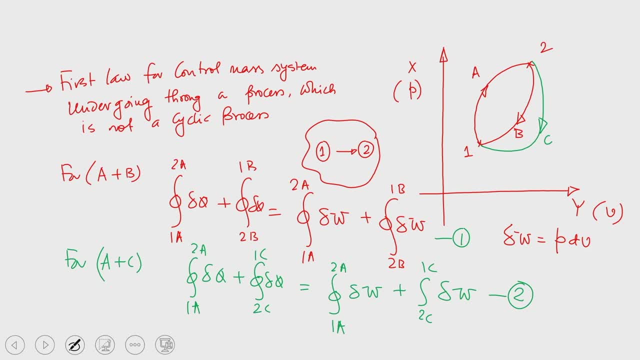 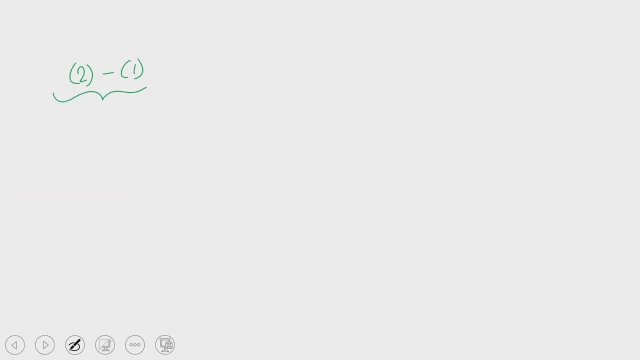 we can do, So we can do this. So what we can do, So what we can do. So what we can do, We can subtract equation 1 from equation 2.. Subtracting equation 1 from equation 2. 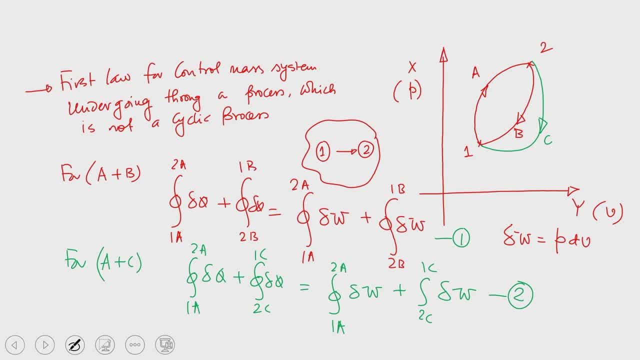 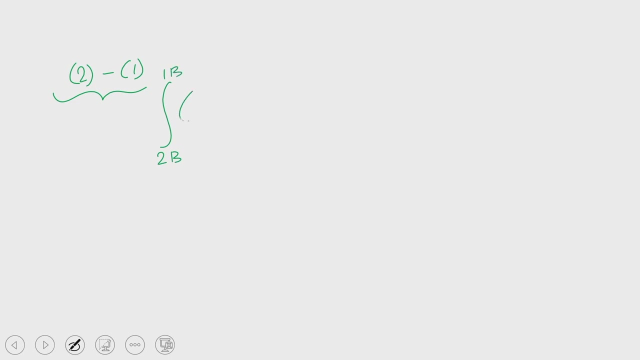 we can write that. we can write what we can write. We can write that 2 b to 1 b del cube equal to. we can write: 2 b to 1 b delta cube minus delta w equal to contour integral. 2 c to 1 c delta cube minus delta w. right, So you? 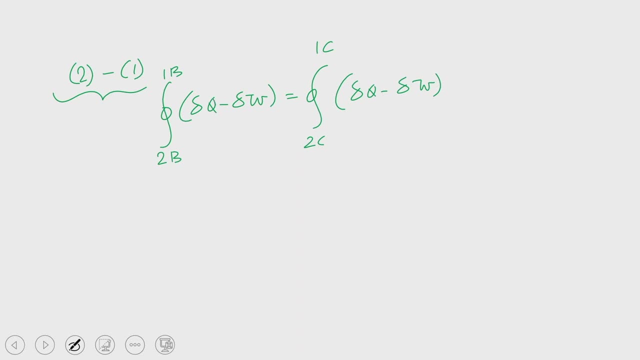 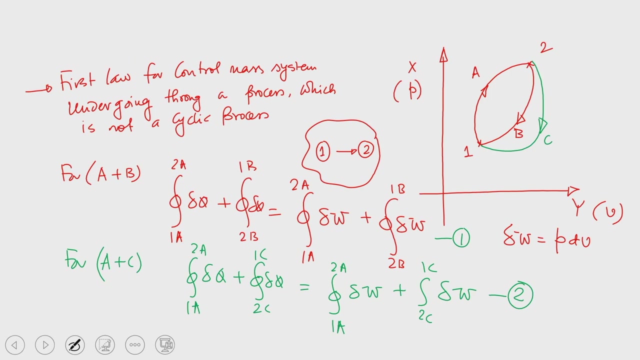 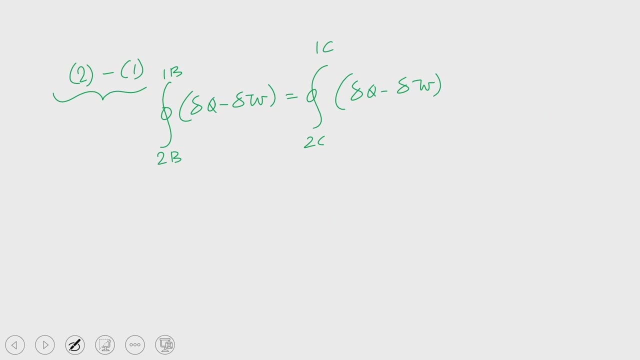 see that we can write if we subtract equation 1 from equation 2.. So now what? because the interaction of feet and walk following the path, following the path, So we can write the following: path a will get cancelled. question is what we can see from this expression though. 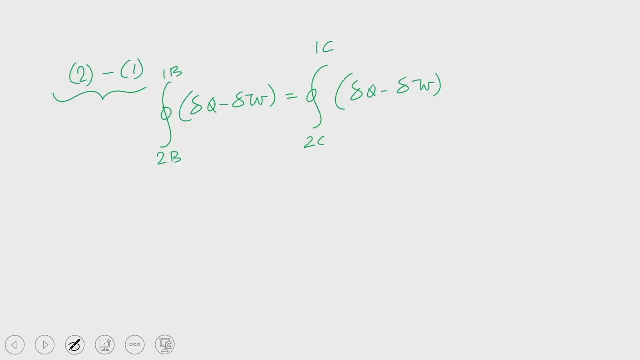 del q and del w. these are path function. So you understand this quantity del q minus del w, though del q and del w they are individually. you know they are path function individually, but the difference of these two quantities is same whether the path is b or c. 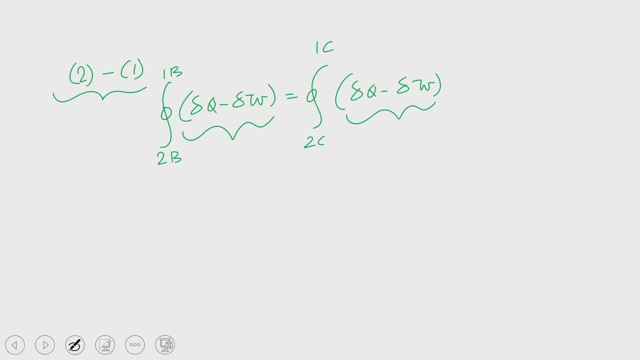 So del q and del w, they are path function individually, but the difference of these two quantities is same whether the path is b or c. The important conclusion from this exercise is that, though del q and del w, they are inexact differential, because I have written 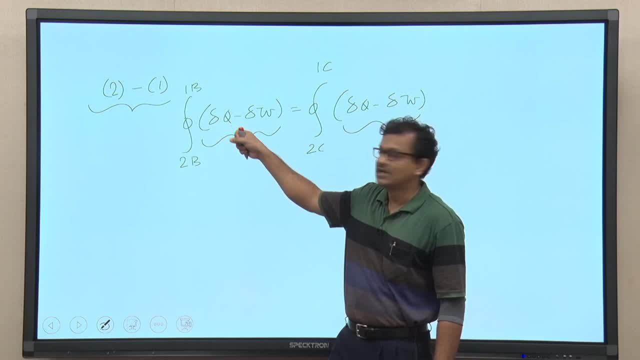 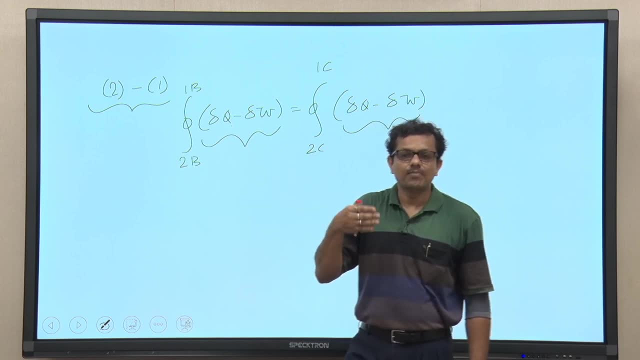 they are not exact, differential, because they are not the point function, they are not the property of the system, So their depends- I mean these 2 quantities- depend on the path through which the process is taking place and the change in pressure and volume following that particular path. So this is basically the process. So you become friends with all. 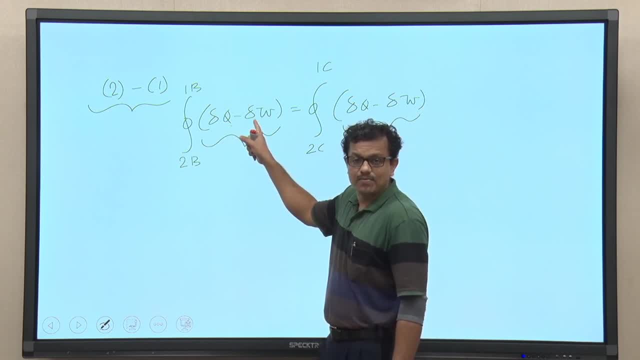 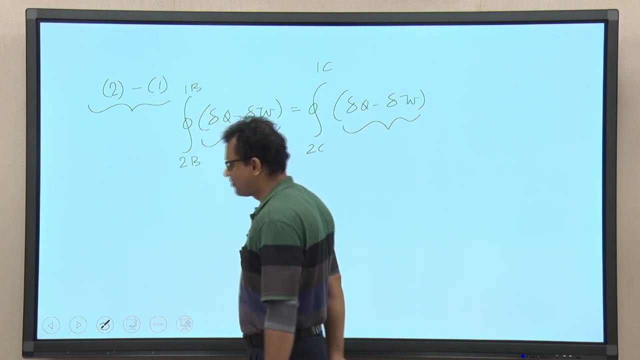 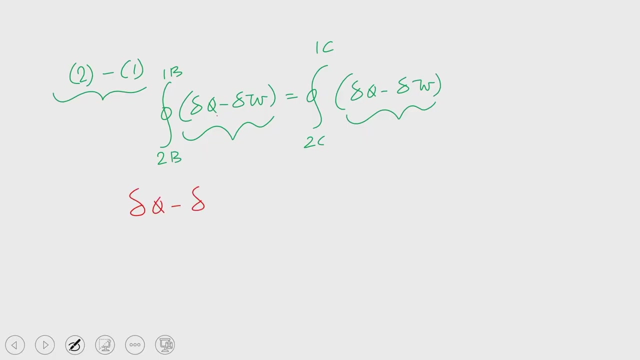 So, though these two quantities are path function individually, but difference of these two quantities does not depend on the path, because you can understand: del Q minus del W, following path 2, following path B, is equal to following path C. So this quantities delta, cube minus. 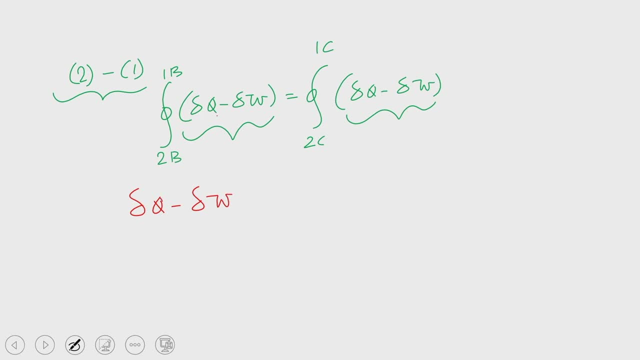 delta W is not the path function. So though delta Q and del W- I mean these two quantities- are path function individually, the difference is not the path function that we can see from this expression now. So this is the property of the system and we write it d, E If the 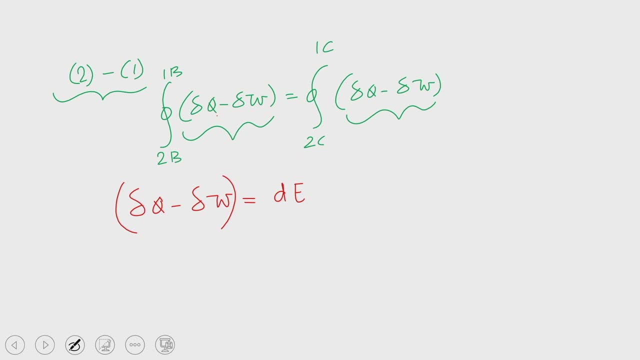 difference between these two quantities is not the path function, that means it is a point function, that is the property of the system. and that is how we could write this: in the form of the differential, in the. in the differential form I mean exact differential form, to be precise. 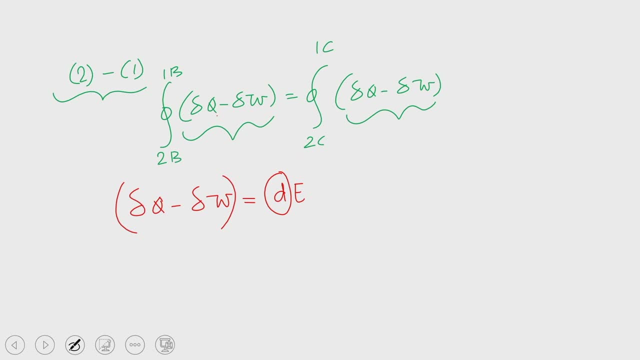 So this is d? E. now, if we try to write one step further, we can write delta cube equal to d? E plus delta Q. So this periods you have studied in your under graduate course. that is the first law: thermodynamics applied to the control mass system and when the system is performing a 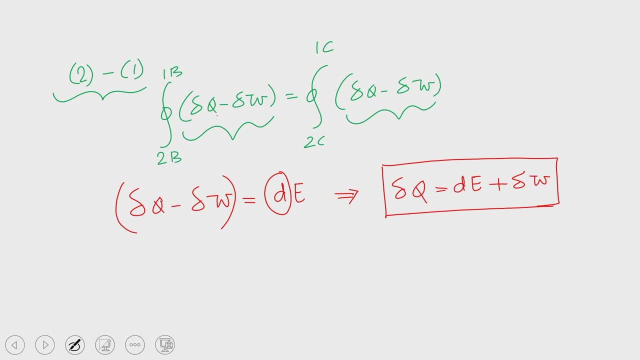 process. the process need not to be a cyclic process. So this is first l of thermodynamics for the control mass system undergoing any generic process related to control mass system. So we have seen this process be a process. would not this be a cyclic process? your, your? process would not be a cyclic process. so this is first l of thermodynamics for the control mass system undergoing any generic process. So the process should be some a thick type of Motor 都. NICHE ebenistona便. Boris здоров nh. princess, Father, now if you write three, you need to write this: 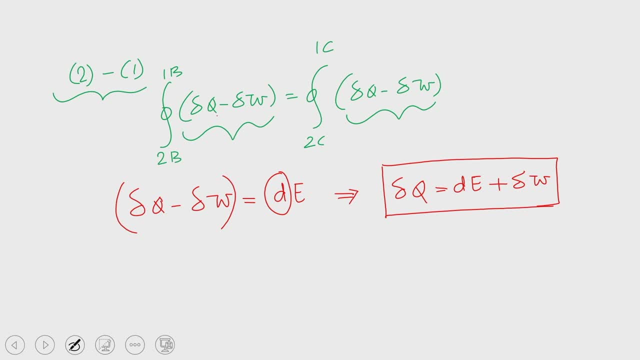 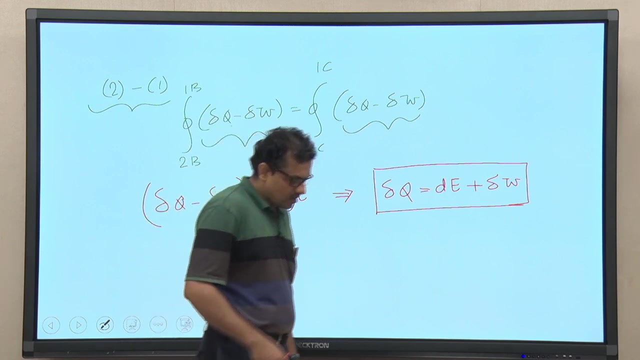 generic or general process. So today, before I complete this lecture, I would like to discuss a few important issues, though those are not, I mean, essential for this particular course, but at least I should discuss, because in the first a few lectures I shall try to discuss about the basic or 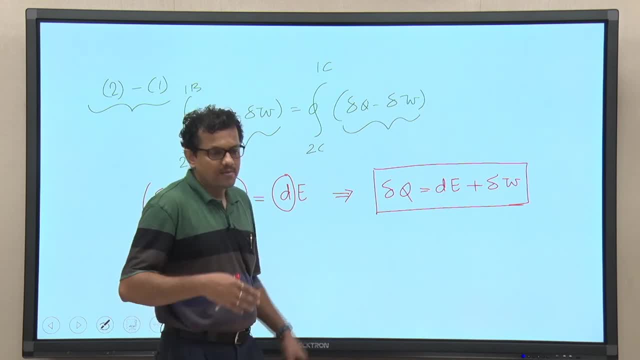 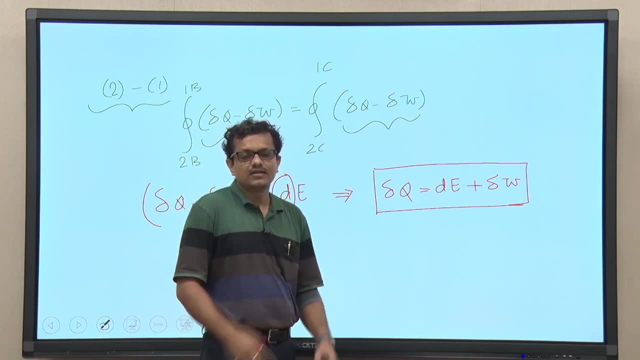 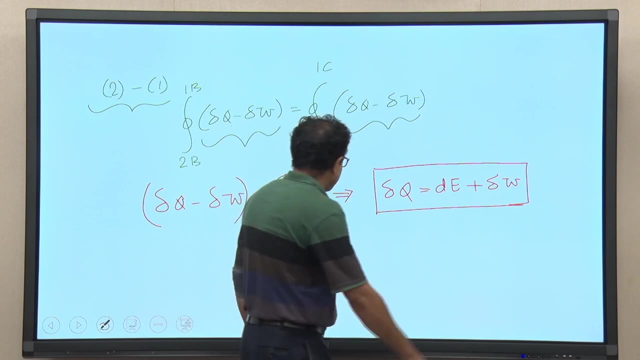 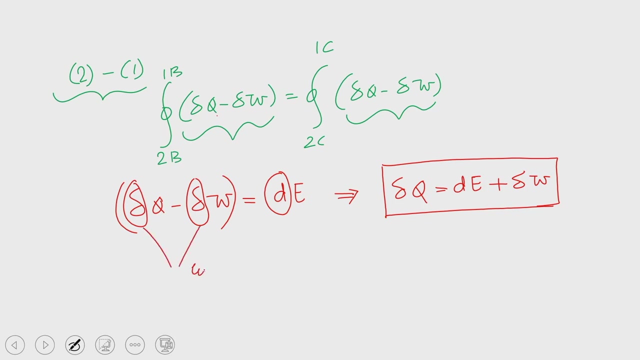 other. I shall try to recap the conceptual part of this: thermodynamics. Why I am discussing- because this will be very much is needed when we will be discussing about different thermal systems- essentially for the quantification of the performance. So you know that these two are the inexact differential. why? because they are path function. 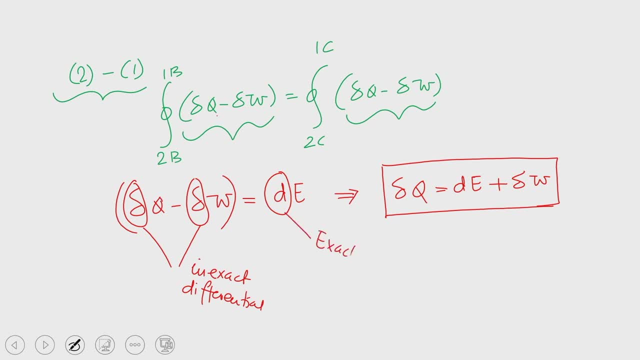 while this is exact differential. So this is a property of the system. because, you know, nice thing to understand, nice thing to see from here is that, though these two quantities are path function individually, but their difference is now the property of the system. 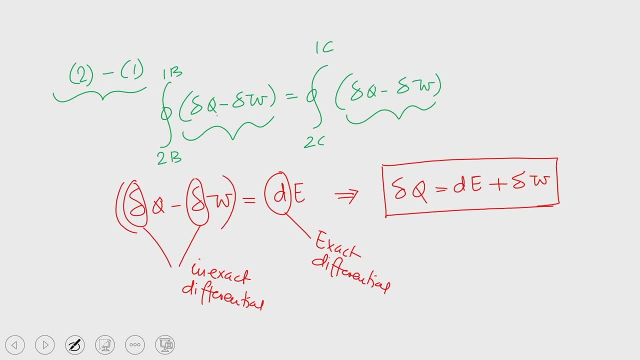 And that is why you would write it in the form of the exact differential. So next, if we try to write that essentially first law of thermodynamics, I am writing first law of thermodynamics, at least for this lecture. from the next class onward, I shall simply write first law, second law, like this: 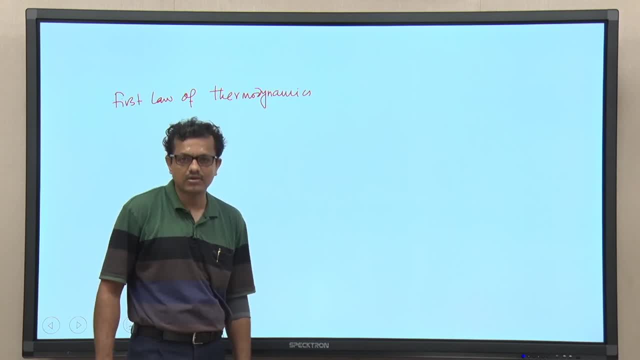 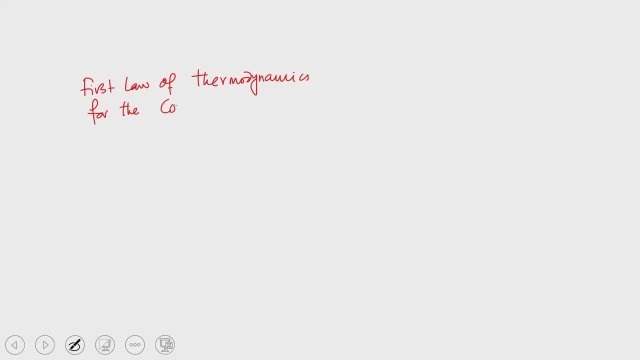 So essentially it refers to first law of the thermodynamics, So first law of thermodynamics for the control mass system undergoing any general processes. So this is So what we have seen from the last slide, that is, delta cube equal to dE plus delta W right. 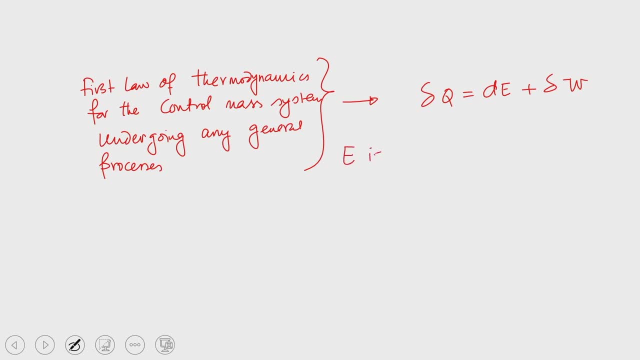 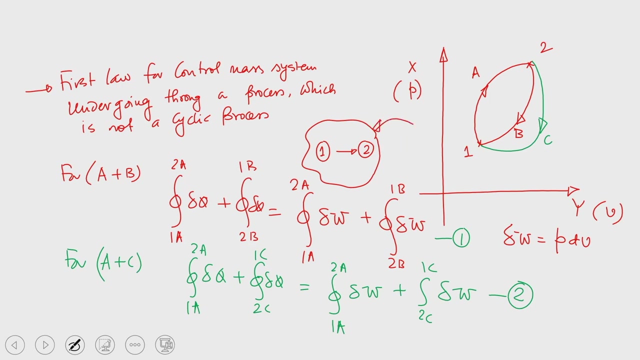 So now here, E is the total energy. So what we have seen from this particular expression. I would like to tell you one important thing. See, that means, if we go back to the slide, So if you supply certain amount of feed to the system, system has rather system holds. 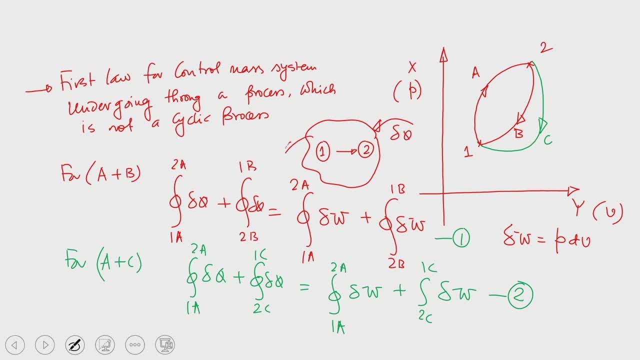 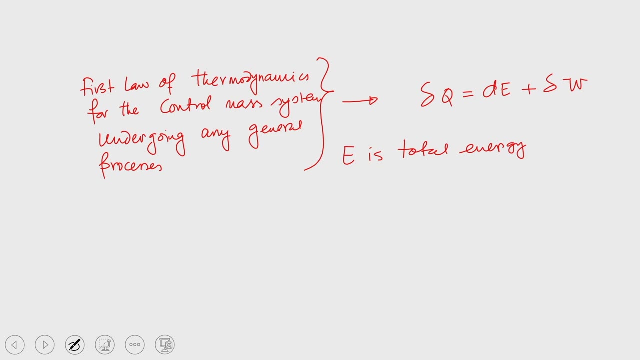 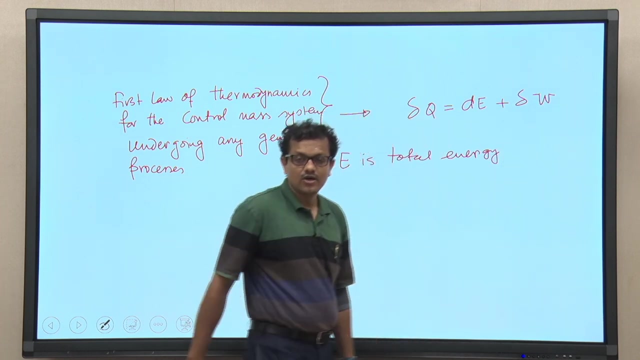 capacity to do some work. right, But try to understand. So if we now look at this particular expression, if we supply certain amount of feed, rather certain amount of energy by heat, to the system, system has capacity or capability to do some work plus. so that means all the energy, all the heat which is being supplied to the system. 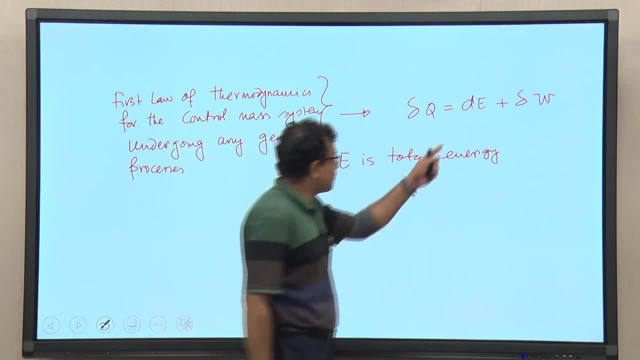 is not getting converted into the work. 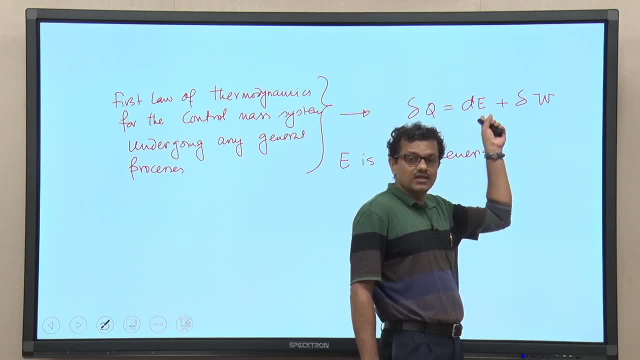 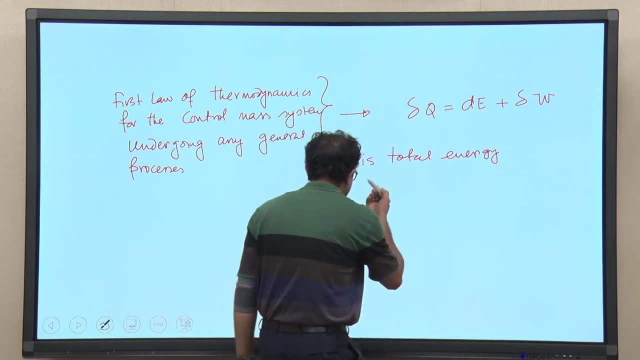 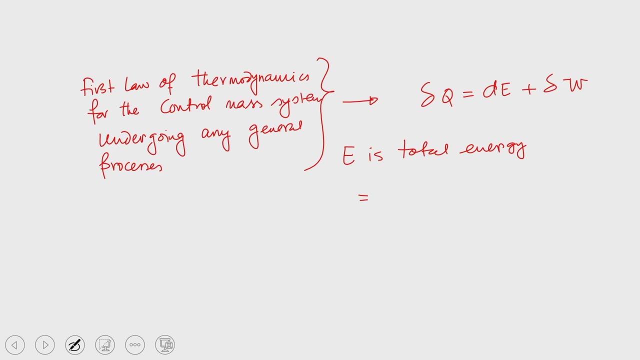 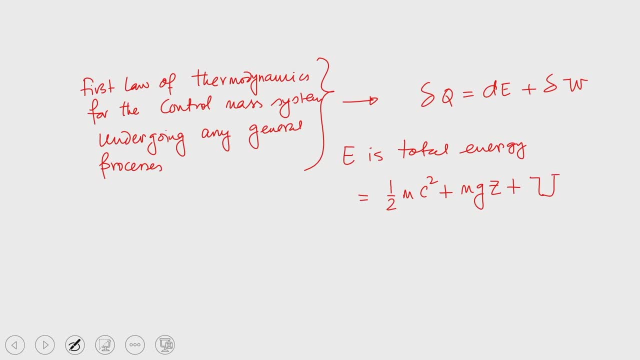 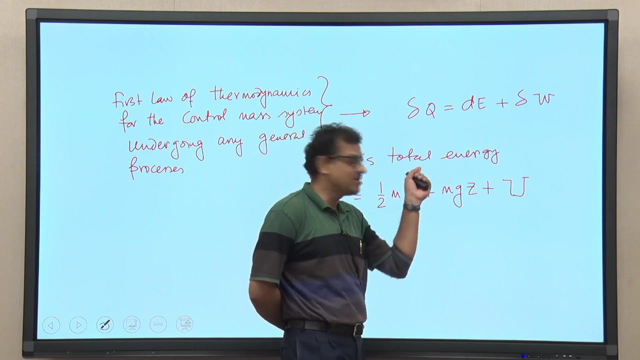 u, that is the. you know one other form. So let me discuss briefly, So you know, the total energy. So that is the remain. I mean it is not possible to have the equal conversion of energy from heat to the work. remaining energy will be there within the system and 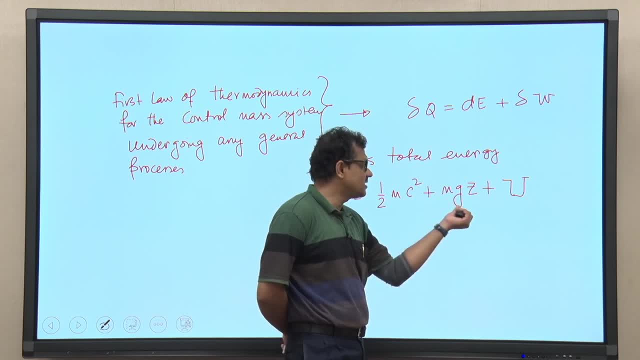 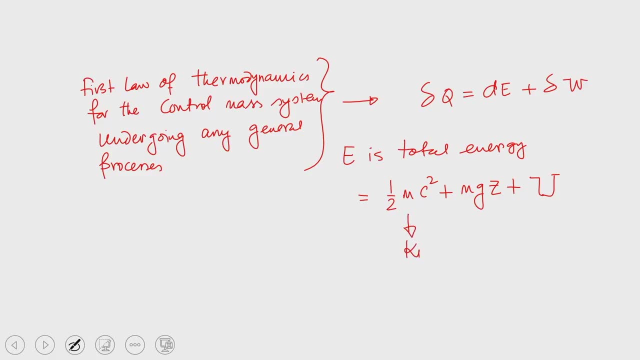 that is nothing but the kinetic energy, potential energy, the form of energy other than this two. So this is the kinetic energy, this is the potential energy, P? e, this is K? e. So now, apart from this two different forms of you know energy, there is another form, and 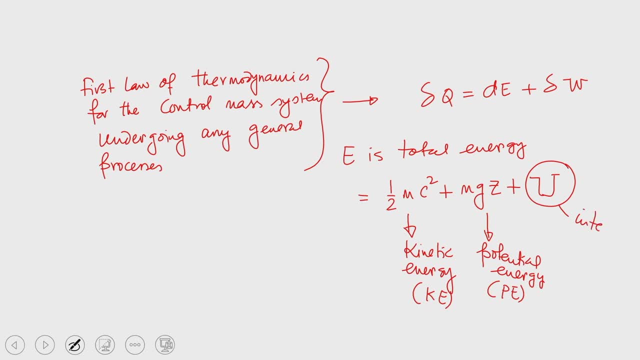 this is known as internal energy. So this is the form of energy other than the kinetic and potential energy. So I am writing: this is another form of energy other than kinetic energy and potential energy, other than the kinetic energy and potential energy, right? So this is very important to understand now. 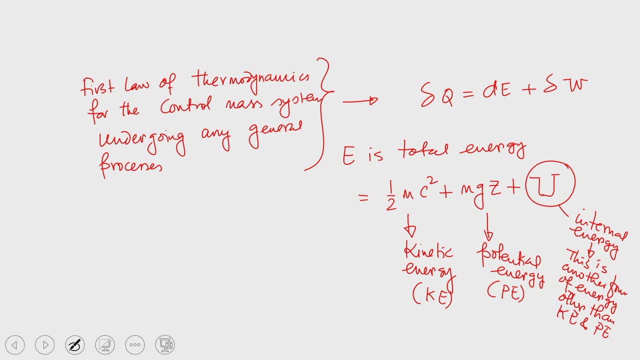 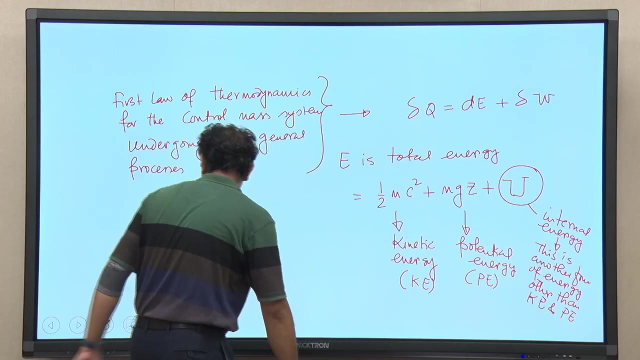 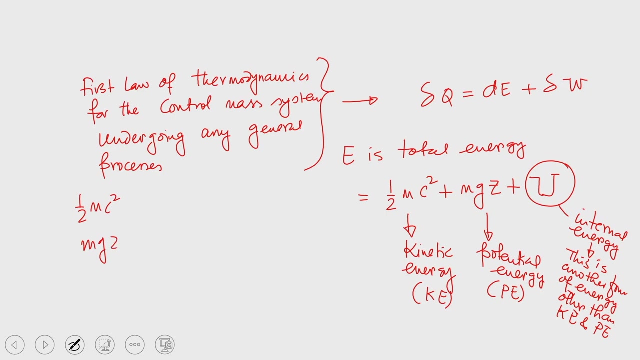 question is in most of these. So basically you know that kinetic energy and potential energy, these two are the microscopic manifestation of the mechanical energy. So basically this half m c square and m g z, So these two, so that is kinetic energy. 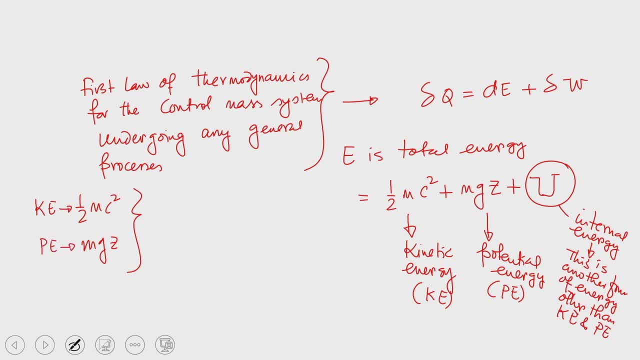 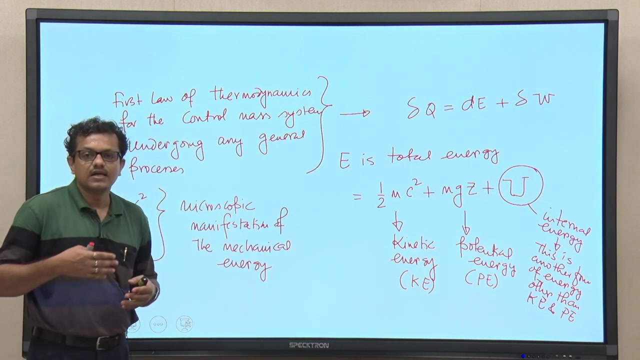 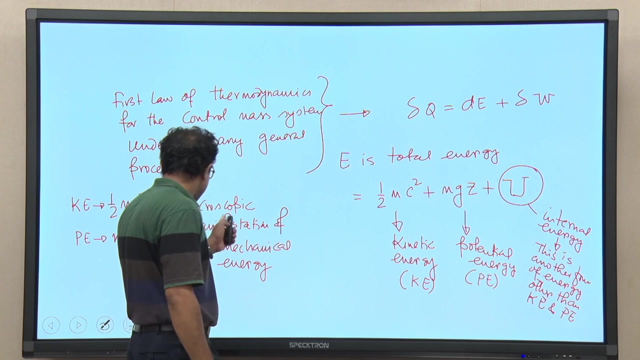 and potential energy. So these two are the microscopic manifestation of the mechanical energy. ok, Where? whereas this phase of the mechanical energy, this phase of the kinetic propeller, is internal energy and that is nothing but the, you know, intermolecular form of energy due to the molecular rearrangement. I will give you an example. So this is microscopic. 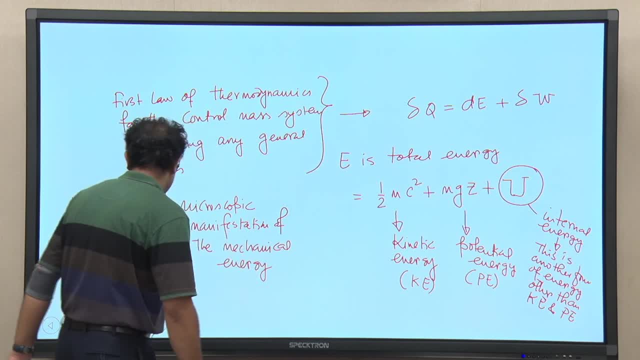 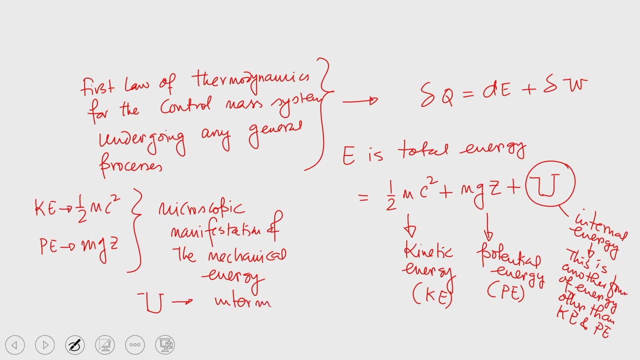 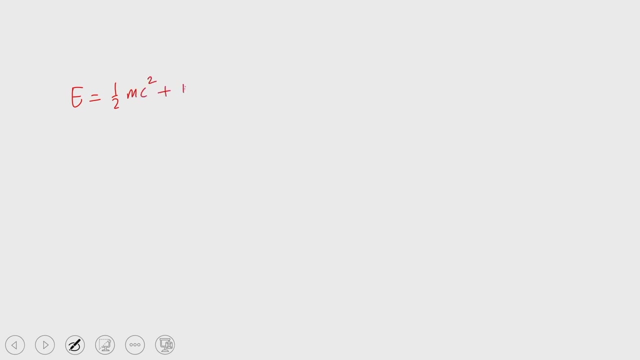 manifestation of the mechanical energy, whereas this u is the intermolecular energy. ok, So U theatre due to the molecular rearrangement. So basically you can write this total energy in terms of the specific energy, because so this E equal to half m c square plus m g z. 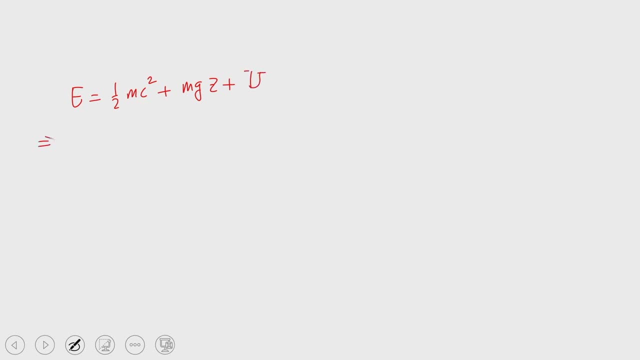 plus total U if we try to write specific energy, So this is the total energy and this is specific energy. E equal to half c square plus g, z plus small u. Now we have discussed already that potential energy and kinetic energy is the microscopic manifestation of the mechanical energy, whereas 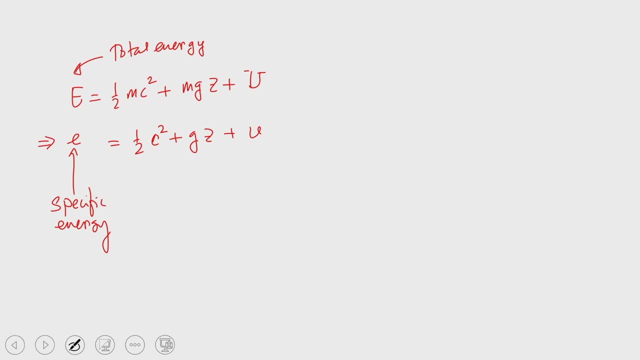 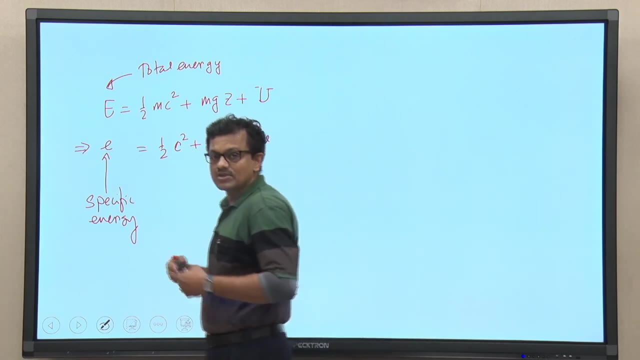 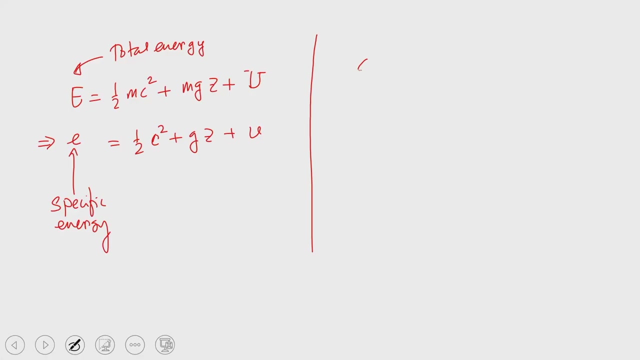 this U, that is the form of energy other than the potential and kinetic energy is the intermolecular energy which is essentially due to molecular rearrangement. So this E equal to half m c square plus m g, z plus U plus delta W In most of the thermodynamic. 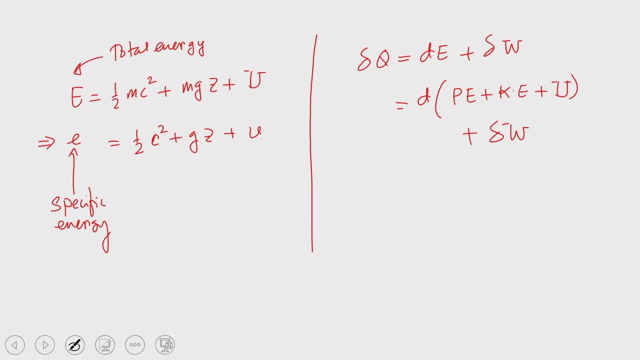 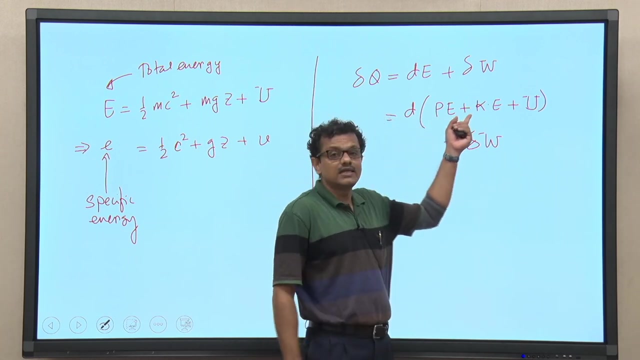 processes, the changes in kinetic and potential energy, is neglected. It is not because of the fact that the it is ignored intentionally. rather, it is seen that in most of the thermodynamic processes the changes in kinetic and potential energy is negligibly small as compared to. 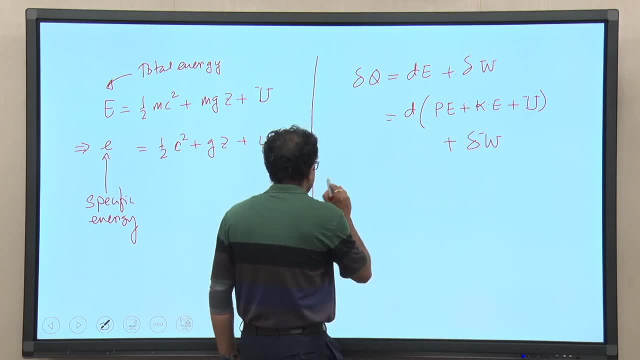 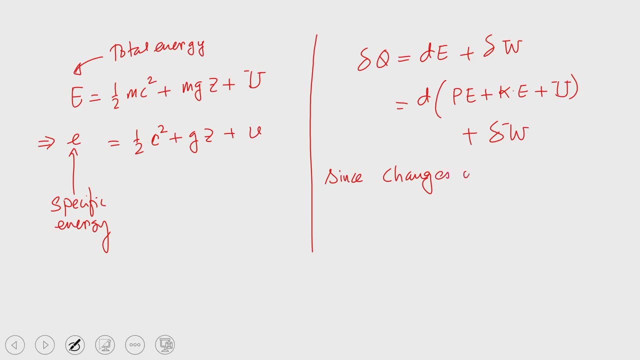 the part which is U. So basically, since changes in PE, here you can write this as the small reflection As shown on picture 2.. This is the local area. So material is very important in the hidroelectric ecology because it controls all the electric. 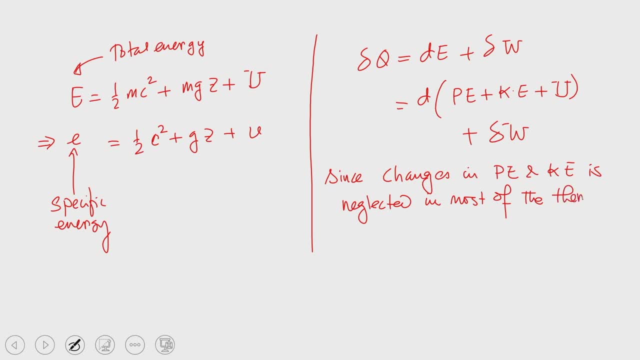 energy used for Woche De, surrounded by austine. So if you look at this graph, the energy is Caesar. The electric gravity is actually equal to 0.14. içinde, By cliche thermodynamic processes we can write delta cube equal to d? u plus delta w. So this is: 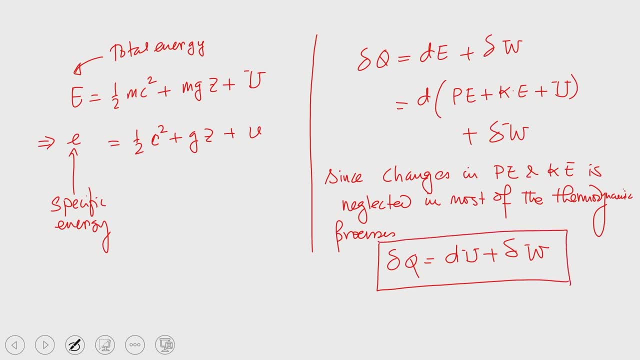 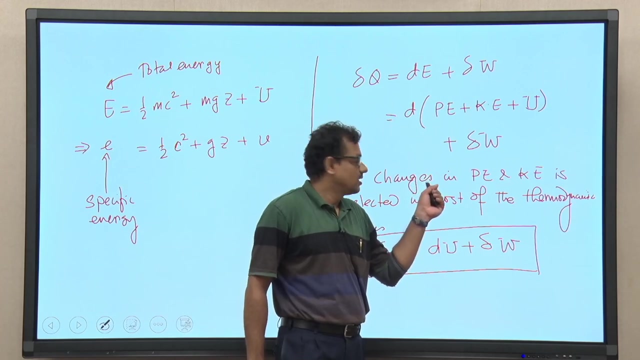 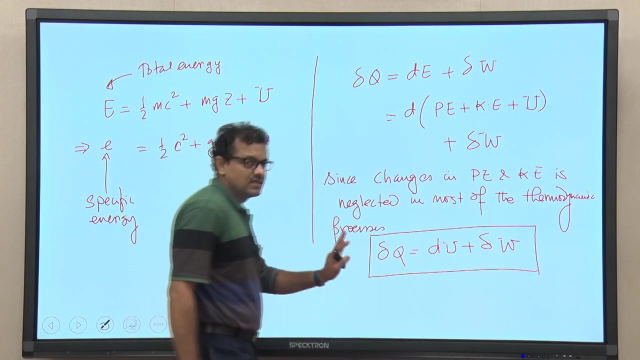 the final form of the first law of thermodynamics for the control mass system undergoing any general process. We could write this form taking this assumption that the changes in potential and kinetic energy is negligible, and what is mostly true for most of the thermodynamic processes. So this is the first law of thermodynamics for the control mass system. 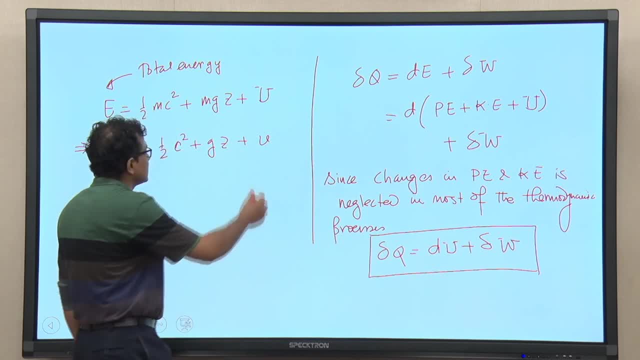 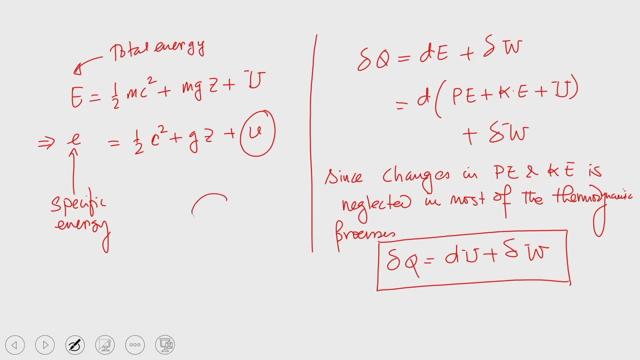 Now question is: I told you one important thing that this fellow is essentially due to the molecular rearrangement. I can give you an example. If you take certain amount of liquid in a container and say the container is like, this container is this, and we are taking, say, water with a few iron particles. 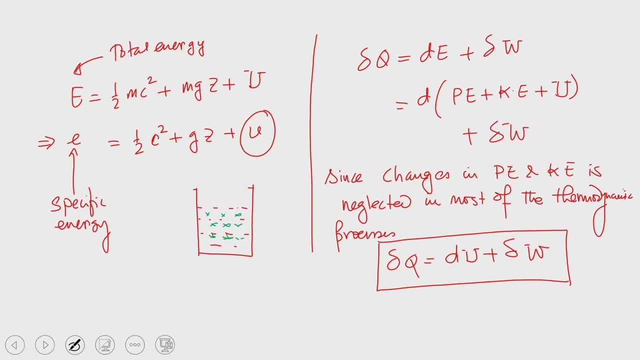 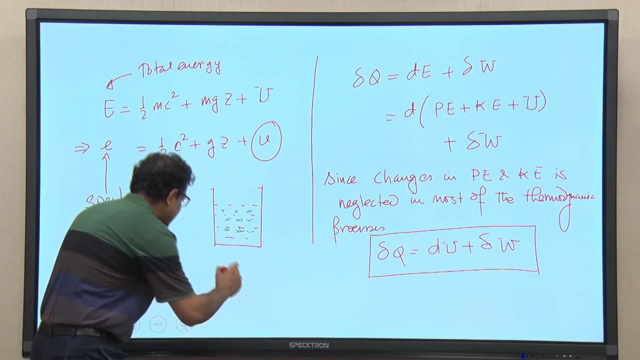 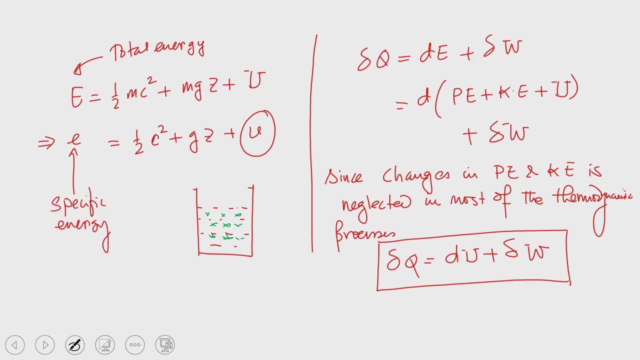 Okay, So this is the container which is containing di water or any water, and a few iron particles are, you know, injected in this liquid. If we have one magnet at the bottom, if we have one magnet at the bottom, say we have one electromagnet E m at the bottom. So this: 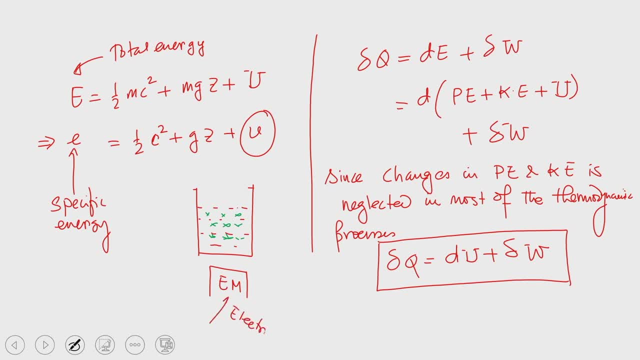 is electromagnet. If we have the electromagnet, then if we energize this magnet by switching on the circuit, then what will happen? All the particles will move towards the bottom of the container and they will remain stored there in When they are remaining stored there. 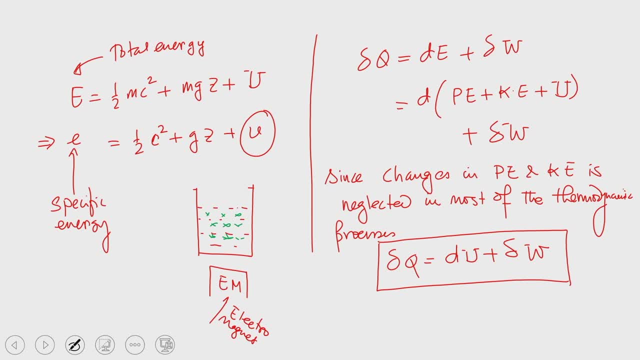 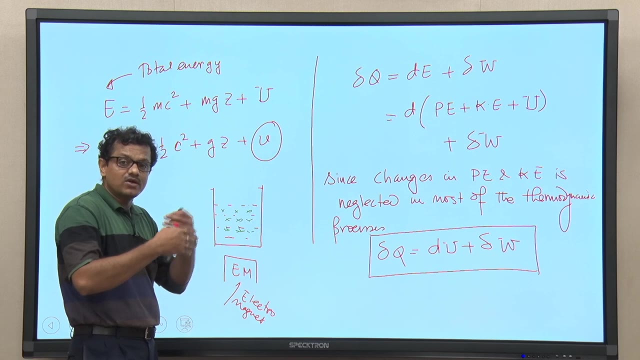 in due to the molecular rearrangement of the total substance which is there in the container. energy will be stored there in. If we switch off the circuit and if we deactivated this electromagnet, what will happen? you know That it is because of the stored energy particles. 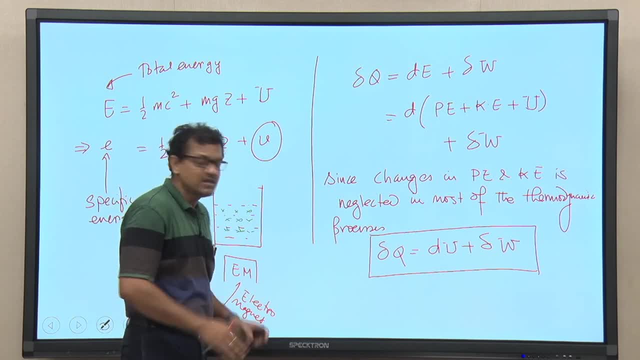 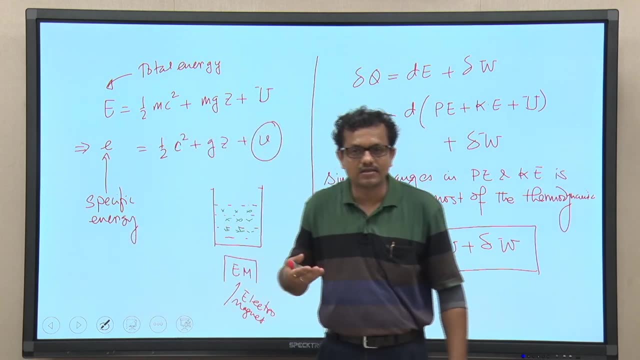 will try to dislodge from the initial positions and they will again slowly come to the original configuration. So this is the concept of the internal energy, So basically other form of the potential and kinetic energy. it is because of the energy, and energy will be. 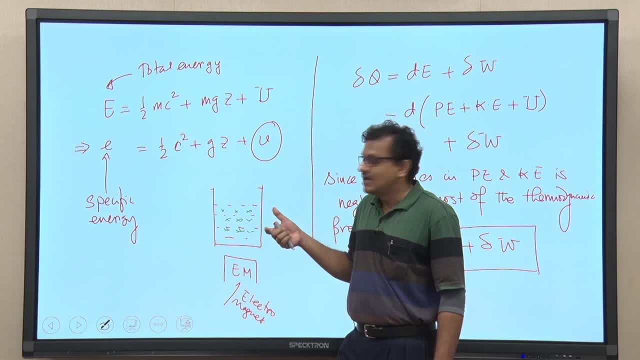 stored there in. If we switch off the circuit and if we deactivate this electromagnet, what will happen? You know that it is because of the stored energy. particles will try to dislodge of the molecular rearrangement. some energy is stored within the system and that is known.